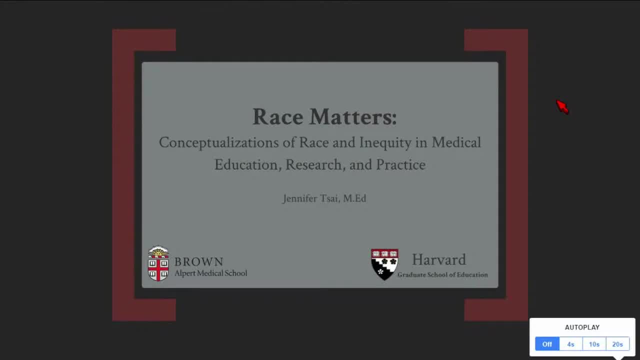 Hi everyone. Sorry, I'm the last speaker. I also want to stop talking as soon as possible, so thank you for sticking with me. I'm not quite a doctor yet, but May 26th catch me with the MD, if I do everything right. 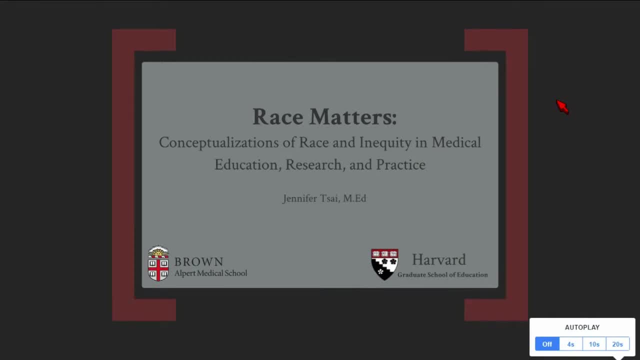 All right. so this topic is not quite directly in line with conversations about institutional diversity. So sorry for the false advertising but I think embedded within it are still really important sort of discussions on structural racial inequity that I hope you'll still find interesting. 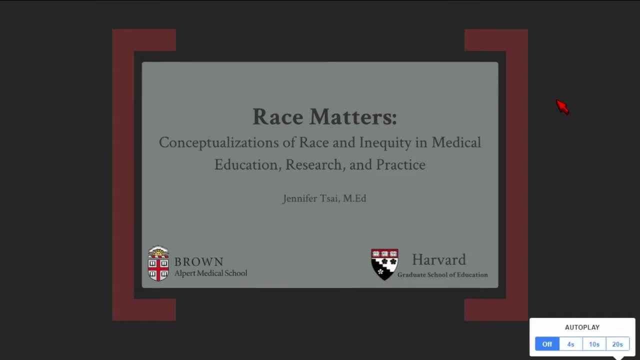 And if you don't find it interesting, you can blame Dr Boatwright, who was so gracious and so kind to extend this invitation to me. So today I'm going to be focusing on the issue of race in medicine, especially how it's been operationalized as a biologic concept. 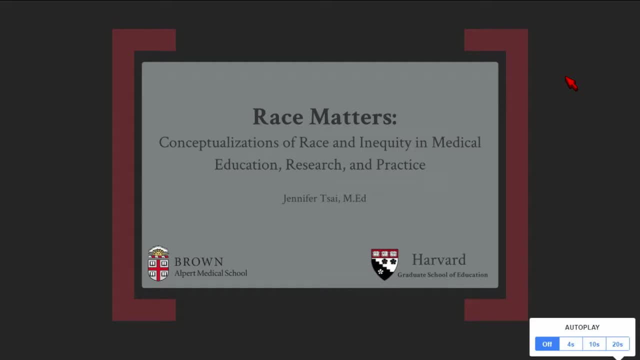 and why, in particular, that's problematic in the way that informs and changes medical education and philosophy. I believe the ways that we imagine and utilize definitions around race is linked to our understanding about racial disparities, health equity and the tools we have to create solutions to those really big problems. 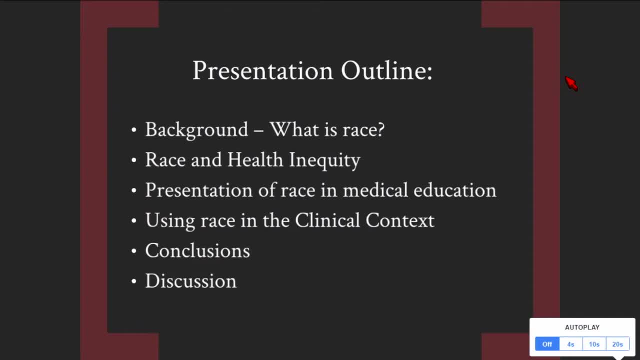 As a presentation roadmap. I'll start by talking a little bit about race as a concept to give background. discuss race as it relates to health inequities. We'll get some examples of how race has been mobilized in medical education and practice. 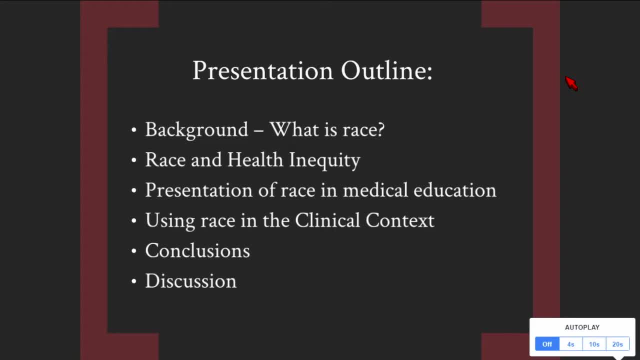 and then talk a little bit about how paying attention to race can be a big part of how we think about health inequities And how race can be both beneficial as well as detrimental, and how to navigate that a little bit. I'll offer some brief conclusions and hopefully we'll have some time for questions. 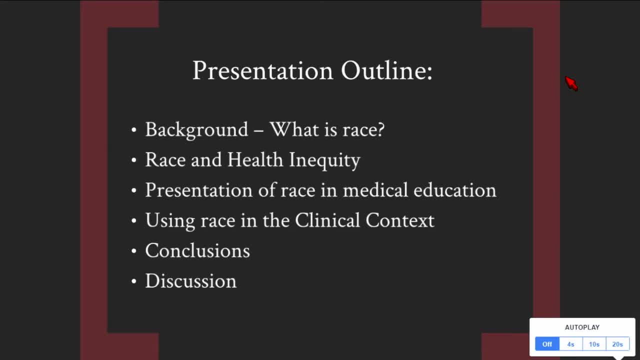 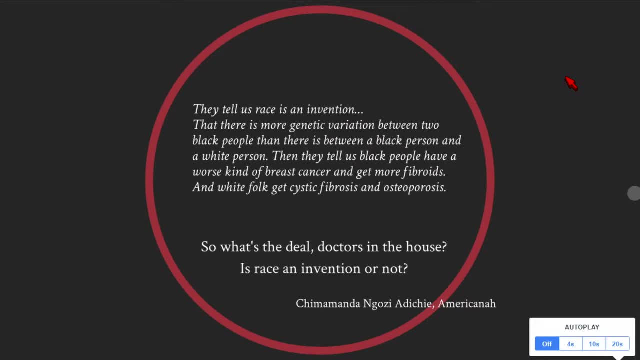 So to begin, I want to bring in a quote written by author Chimimanda Ngozi Adichie In her best-selling book Americana. she writes: they tell us race is an invention, that there is more genetic variation between two black people. 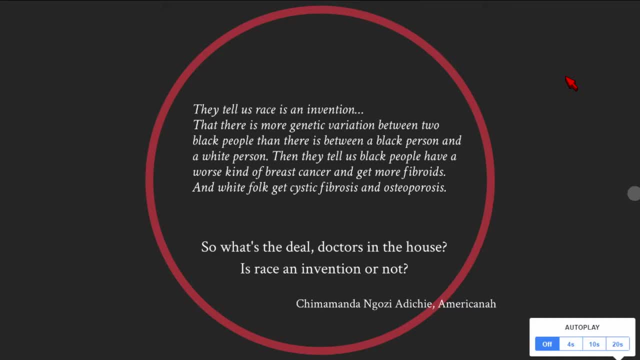 than there is between a black person and a white person. Then they tell us black people have a worse kind of breast cancer and get more fibroids, and white folk get cystic fibroids. So what's the deal? doctors in the house. 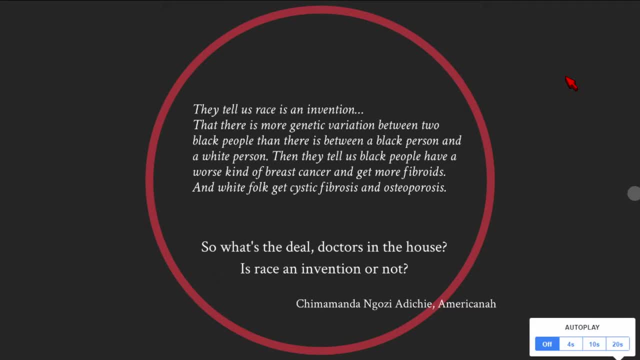 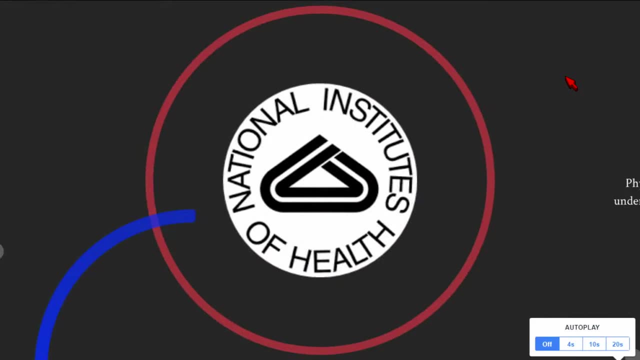 Is race an invention or not? Race seems to matter in medicine And in 1993, the National Institute of Health passed the Revitalization Act which actually mandated that data on racial minorities and women be included in all funded research. The problem is, while this Revitalization Act now requires scientific research to include these categories, 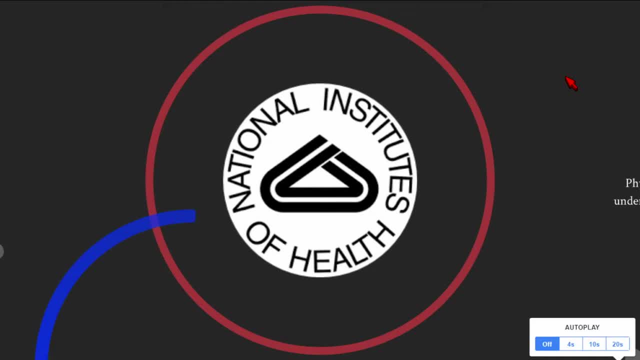 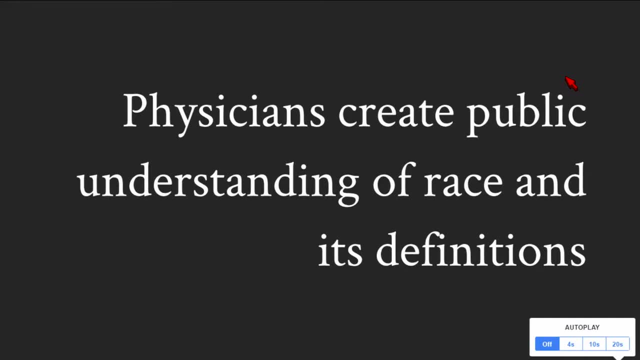 very few scientists and doctors have actually studied the complexities of racial politics in the United States. Though physicians are ill-acquired, equipped and not at all trained in racial formation theory, they are huge players in creating public understanding about race, as well as its definitions. 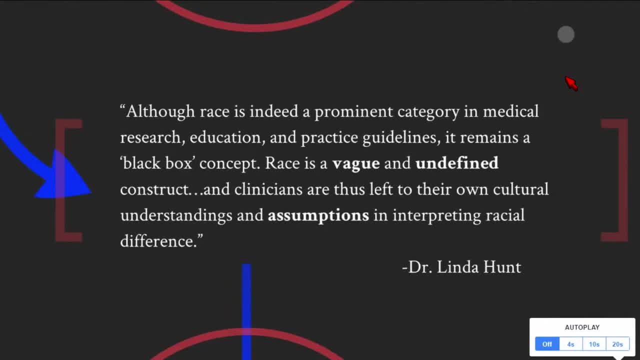 This is summed up by Dr Hunt, who writes: although race is indeed a prominent category in medical research, education and practice guidelines, it remains a black box concept. Race is a vague and undefined construct, and clinicians are thus left to their own cultural understandings and assumptions in interpreting racial difference. 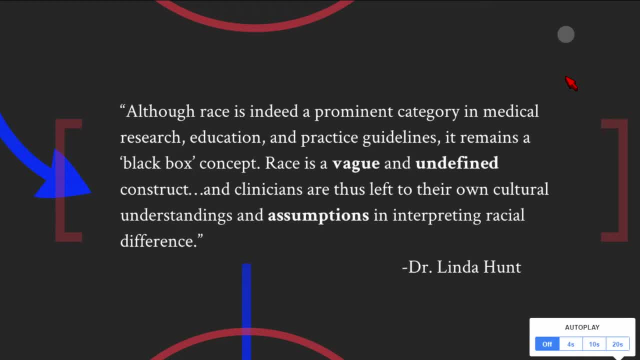 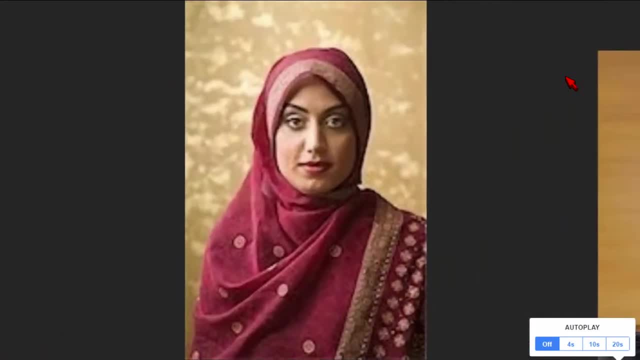 So to understand how we should use race in the clinic, we first have to answer this fundamental question: What is race? According to the US Census, this woman is Caucasian. These two women are twins, as are these two toddlers shown here, with their shared biologic parents. 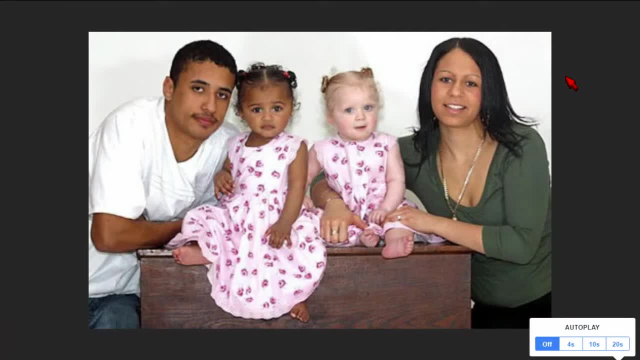 Dorothy Roberts is a biracial legal scholar who talks about race very often, and she makes the point of describing herself as a black woman with a white father rather than a white woman with a black mother. So these are essentially two sides of the same exact coin. 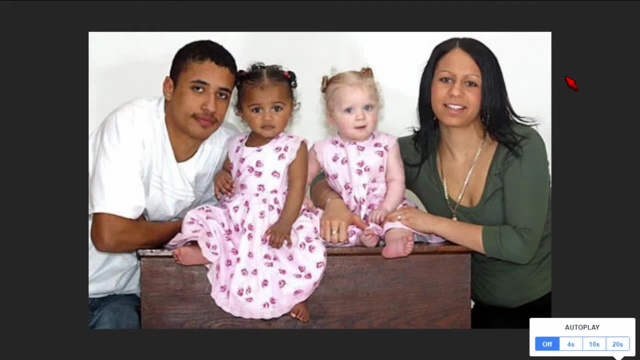 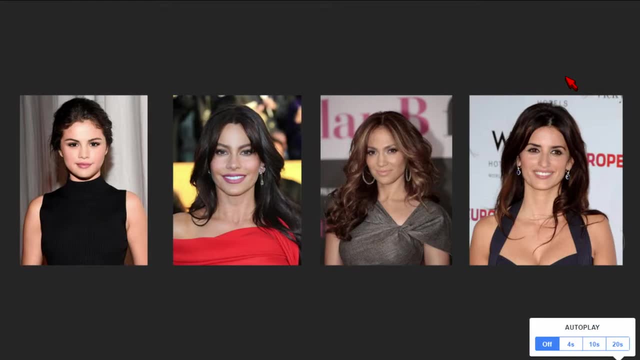 and yet why does one of those make so much more sense? If we look at these women's races as it is used in clinical research, we would group them into a single patient subset- Hispanic-Latina women, and make assumptions about what that might mean for their clinical care. 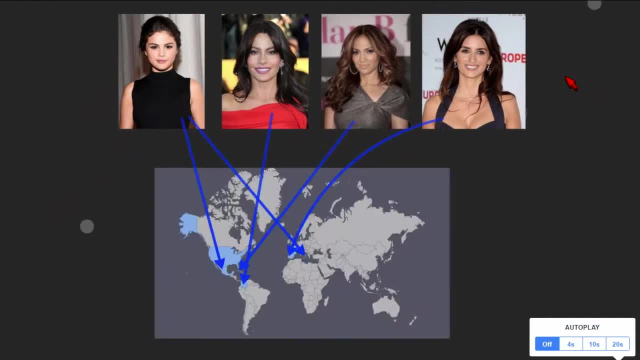 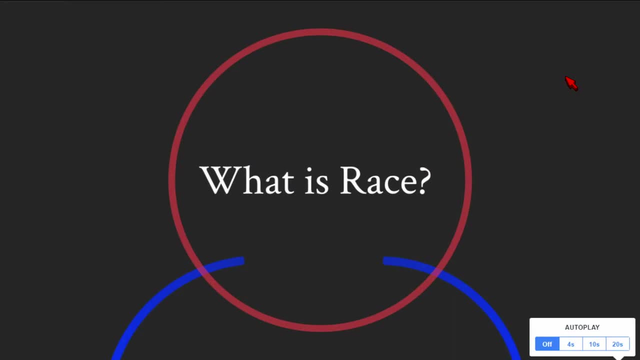 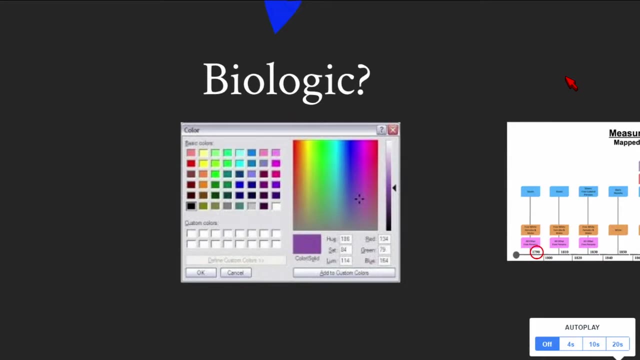 But these women are from Mexico, Italy, Colombia, Puerto Rico and Spain, So race itself really is not a biologic category. Genetic variation is continuous and overlapping among populations, yet medical discourse and research often treat racial groups as discrete, immutable and genetically homogenous. 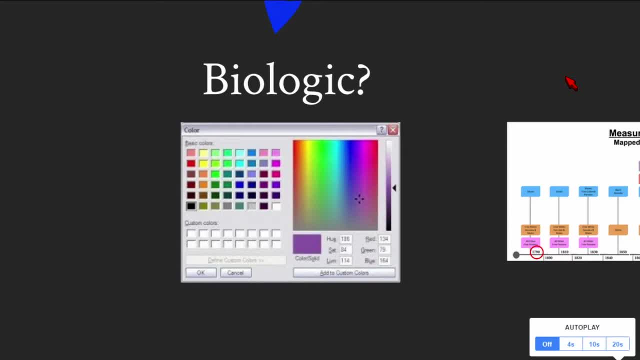 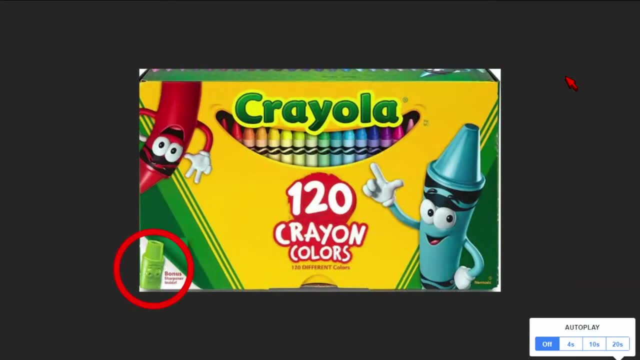 In some ways it's like asking us to limit ourselves to this dinky Crayola 8-pack when you know, all the cool kids have the 120-pack with the built-in sharpener at the back. I'm still pretty bitter that my parents didn't buy this for me. 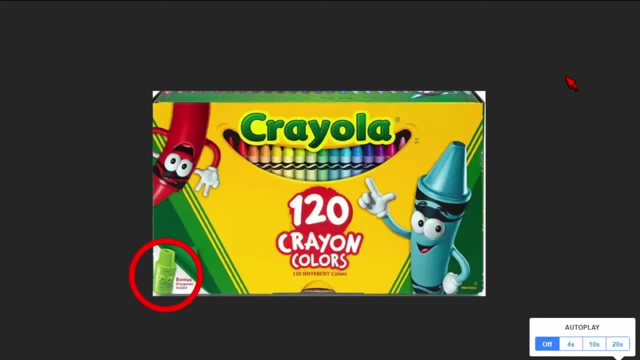 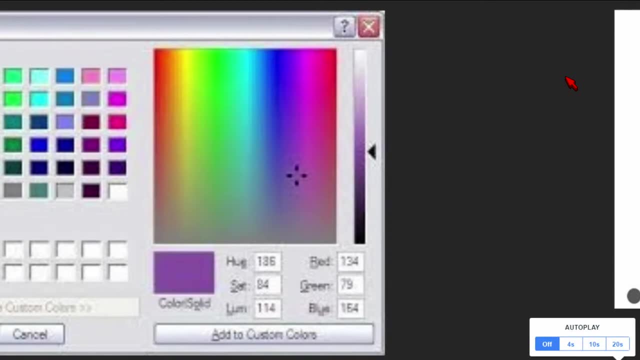 so I'm going to keep mentioning it. So in reality, it's actually more accurate to visualize the idea of genetic variation using a spectrum that mimics clinal variation. But even still, using this idea of clinal variation and genetic diversity is not enough to define and reproduce our notions of race. 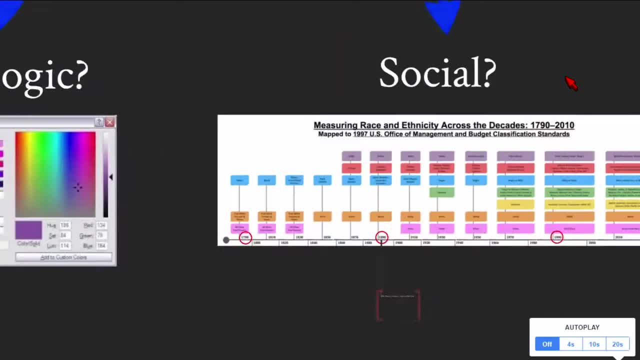 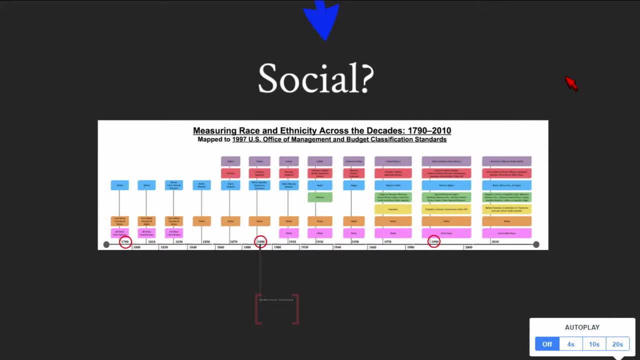 In actuality, racial categories are sociopolitically constructed and therefore dynamic, fluid and transient. If you look at the entire history of the US Census, for example, it has changed every decade since 1790.. And looking closer at this evolution, 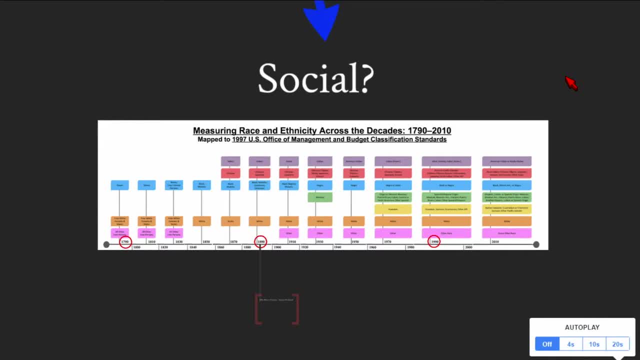 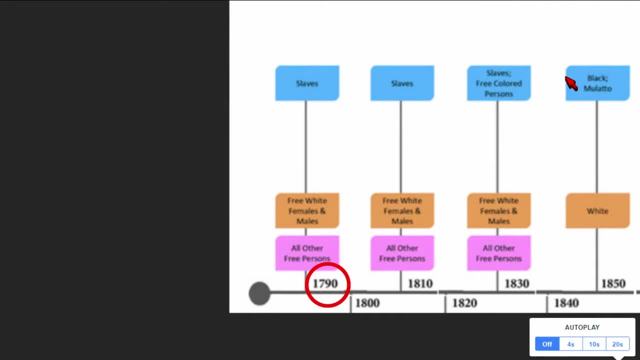 helps us really clearly dismantle this biologic idea of race. In 1790, the racial categories included in the US Census were slaves, free white females and males and all other free persons. So also pay attention to free being a part of racial definitions. 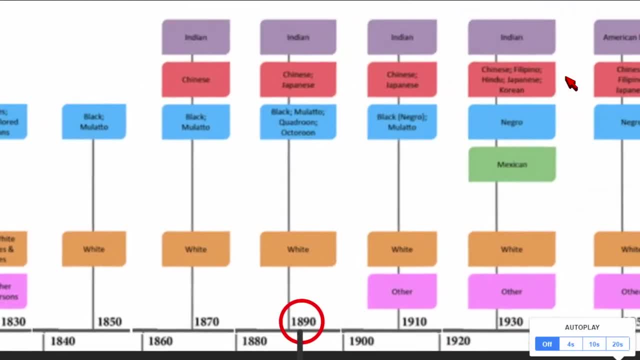 In 1890, the Census included a category for Native Americans, representing the first attempt of the government to catalog American Indians, Chinese, Japanese, due to a rapid influx of migrant workers from Asia. white and a black subcategory that included distinctions for mulatto. 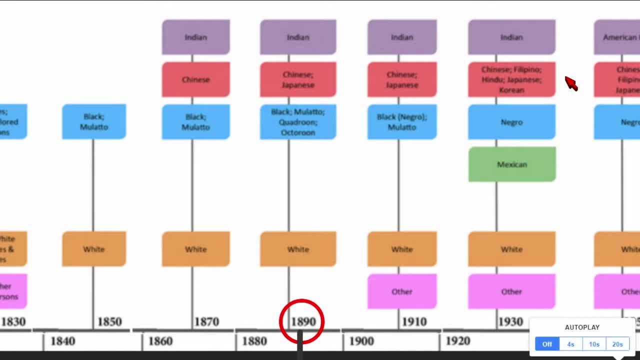 quadroon and octoroon. So these terms, now derogatory, denote people who are one-half, one-quarter or one-eighth black. And these labels are really born out of anxiety. They're born along this idea of the one-drop rule. 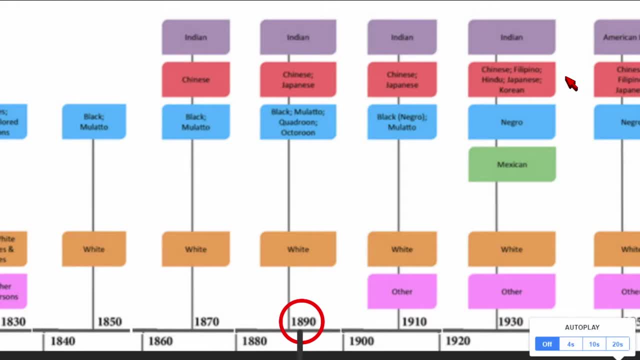 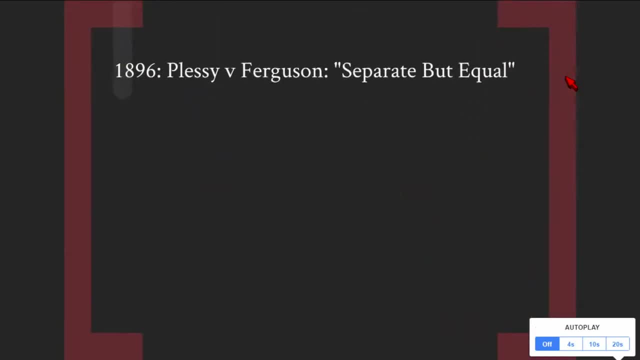 which is heavily mobilized in conversations around legal citizenship and legal rights. In 1896, the landmark case of Plessy v Ferguson declared the jurisdiction of separate but equal. But we forget that the initiation of this legal battle, a major argument of Homer Plessy's, was the fact that, as a free man, 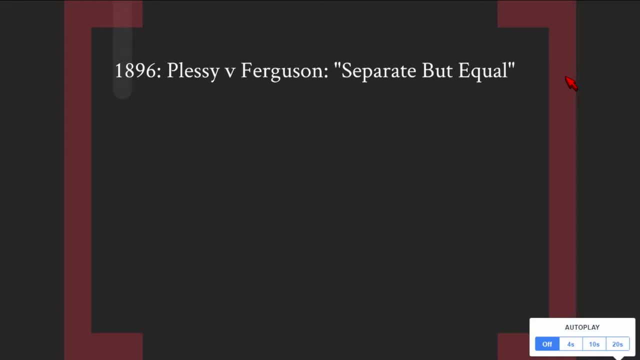 as an octoroon. as a man who's only one-eighth black, he was white. The court decided that if Plessy was a white man, he had a valid case and could have his quote action for damages from the company for being deprived of his so-called property. 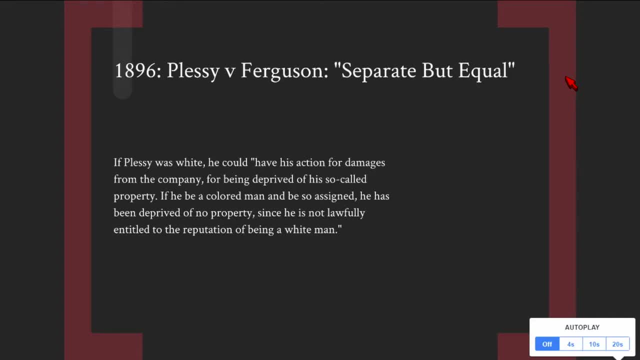 If he be a colored man and be so assigned, he has been deprived of no property since he is not lawfully entitled to the reputation of being a white man. History shows us how important it was for the courts to determine who was white and who was not. 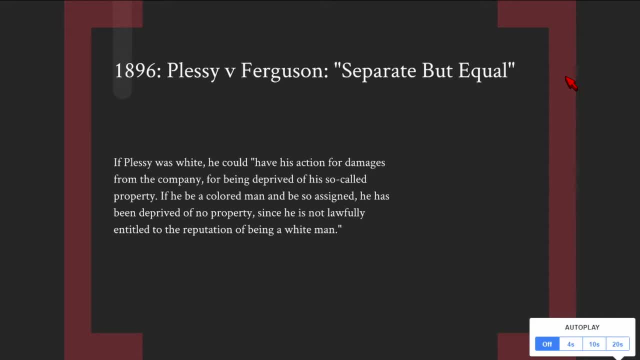 So race began as a legal definition, not a matter of genes or internal construction. And amidst lawsuits demanding rights for property interest in the 1900s, the courts came up with rulings that decreed- quote: a white person has been held to include an Armenian-born. 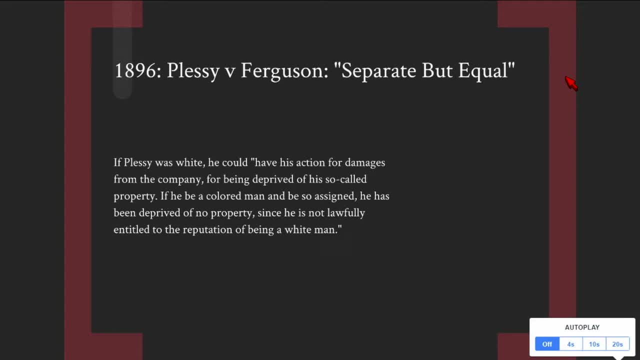 an Armenian-born in Asiatic Turkey, a person but of one-sixteenth Indian blood and a Syrian, but not to include Afghans, American Indians, Chinese, Filipinos, Hawaiians, Hindus, Japanese Koreans, Negros. Nor does a white person include a person having one-fourth of African blood. 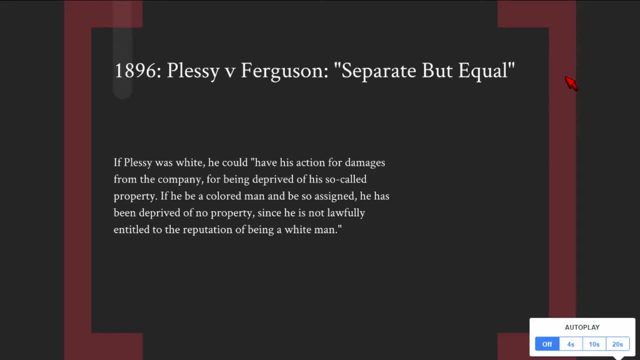 a person in whom Malay blood predominates, a person whose father was a German and whose mother was a Japanese, a person whose father was a white Canadian and whose mother was an Indian woman, or a person whose mother was a Chinese and whose father was the son of a Portuguese father and a Chinese mother. 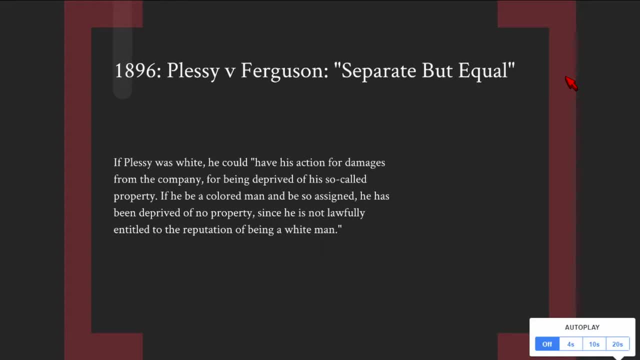 Okay, so whiteness is not simple and it's not biologic and it's not genetic, and this is really demonstrative of that. A hundred years after the Plessy v Ferguson ruling in 1990, the US Census expanded to include a greater number of nationalities. 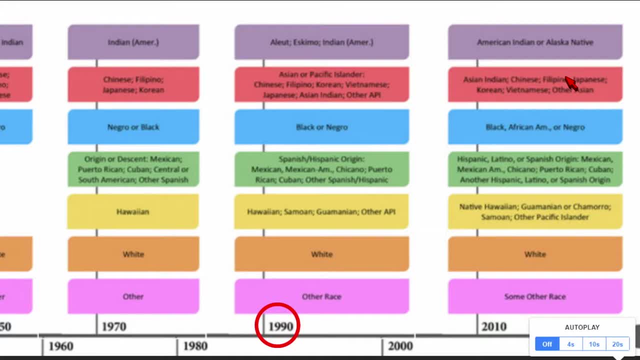 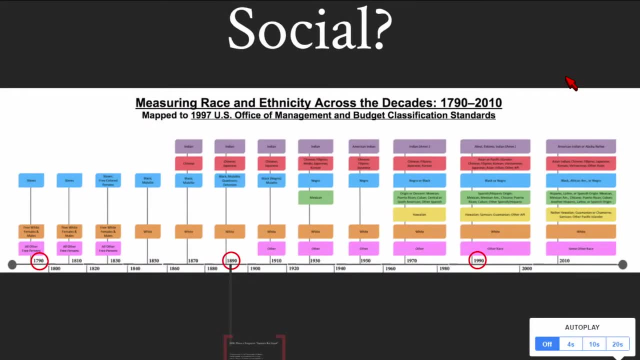 that continue to be grouped under these broad swaths that we recognize from medical research. So our understanding and the official lines of race have been drawn and redrawn over and over again, based on shifting understanding of citizenship, blood respectability, heritability, as well as color. 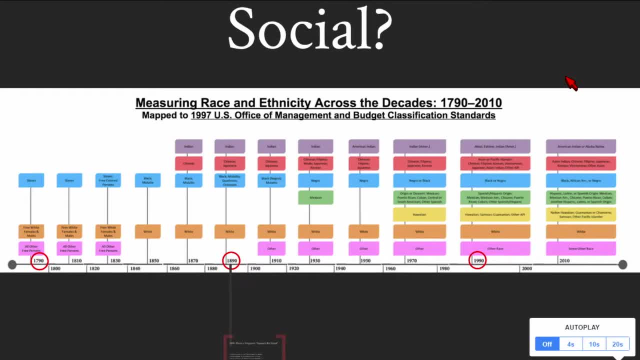 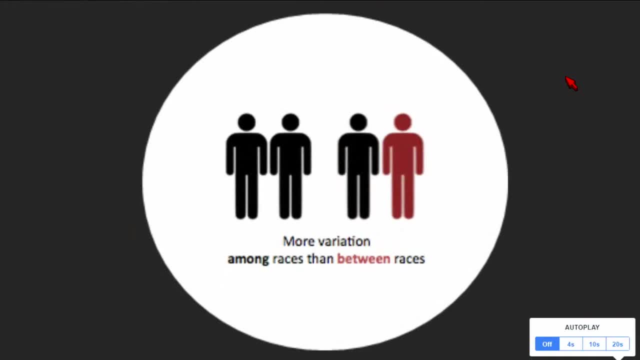 Race is a government-produced category instead of a static genomic entity. Studies have demonstrated, as Adichie mentions, that genetic differences are statistically higher within racial groups than between racial groups. So it's a little bit counter-intuitive, but indeed statistically there's less genetic overlap. 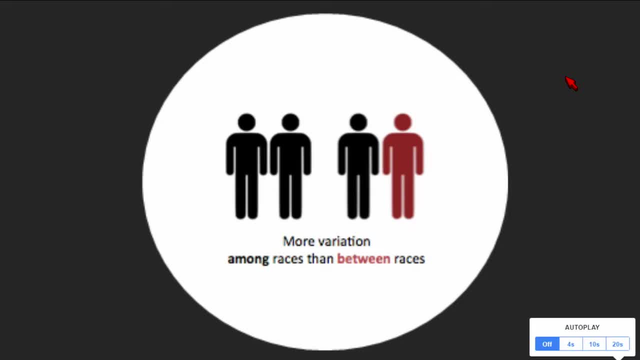 between two unrelated black patients waiting in your clinic waiting room than between one of those black patients and a white neighbor. To be clear, ancestral alleles can affect disease rates and pharmaceutical efficacy, but these alleles do not align neatly with commonly used racial groupings. 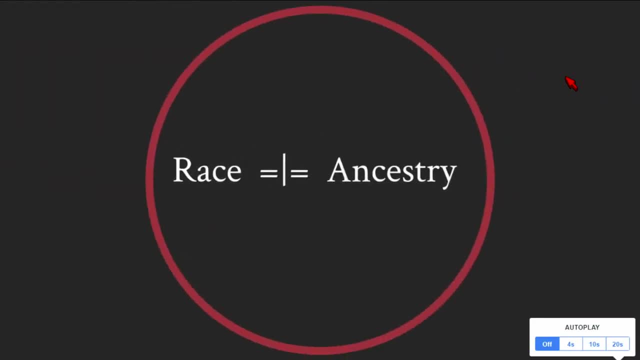 And this is important- Reductive race categories cannot be substituted for genetic ancestry and indeed are very poor proxies for biologic markers. Our understanding of race is not a good indication of family history. Add to this the consideration that, in recent studies, physicians inaccurately classified the race of over 50% of their patients. 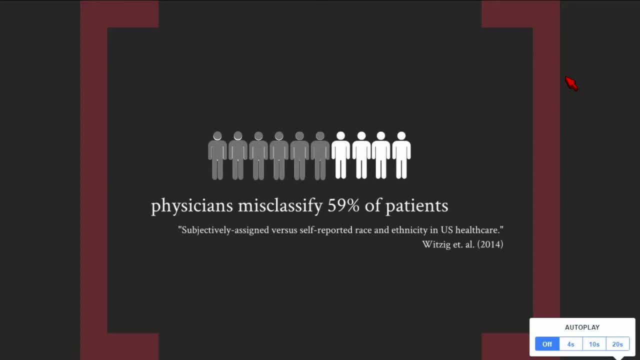 It becomes clear that physician evaluation of skin color phenotypes seeks to make medical decisions off of decidedly non-scientific metrics, As Dr Hunt mentions. because medical education rarely addresses this concept explicitly, healthcare providers are left to formulate their own understandings. 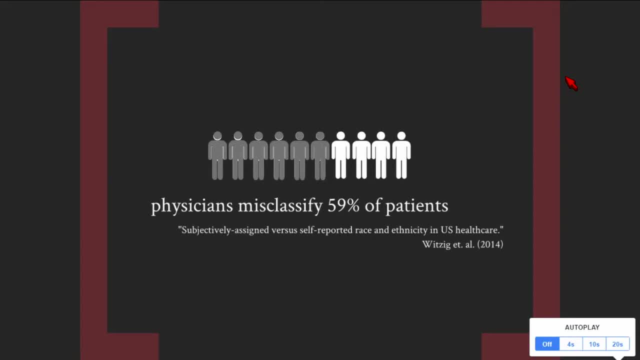 of its legitimacy in the clinic. Now, this is not to say race doesn't matter. Race has a very significant impact on people and their health. This impact, however, is not necessarily written into DNA, but engendered through social inequities. 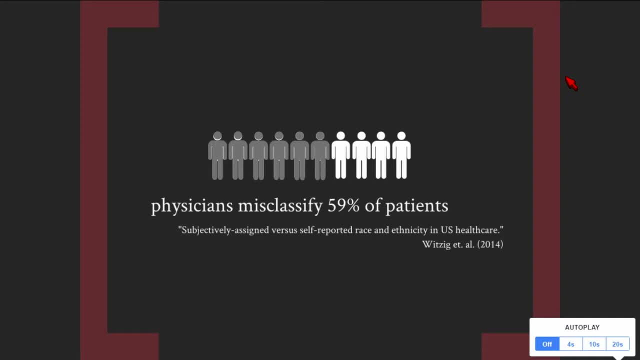 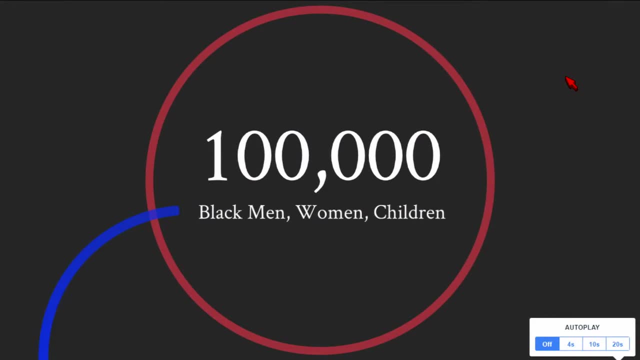 caused by a legacy of discriminatory policies and institutions in this country. Every year, more than 100,000 black men, women and children die because their mortality rates do not equal that of their white counterparts. This statistic means that if the disease and mortality rates for black people 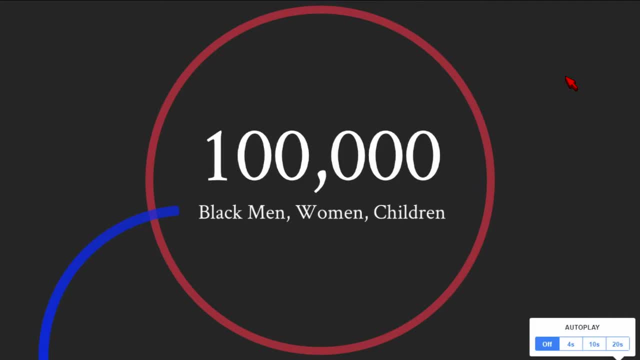 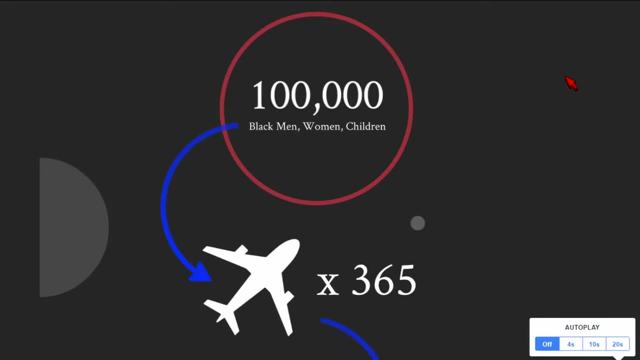 were the same as they are for white people, we would stop the equivalent of a jumbo jet carrying 260 people from crashing every single day. We see staggering disparities in heart disease, cancer, stroke, diabetes, severity, mortality and more. 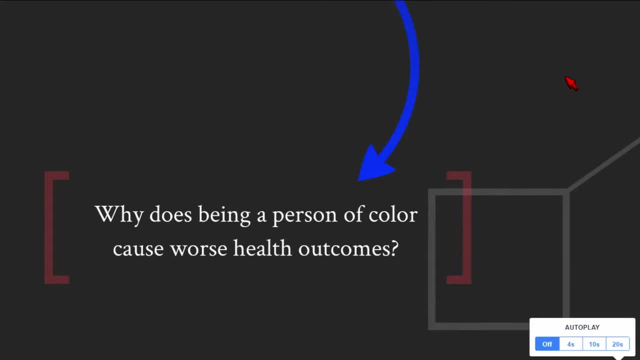 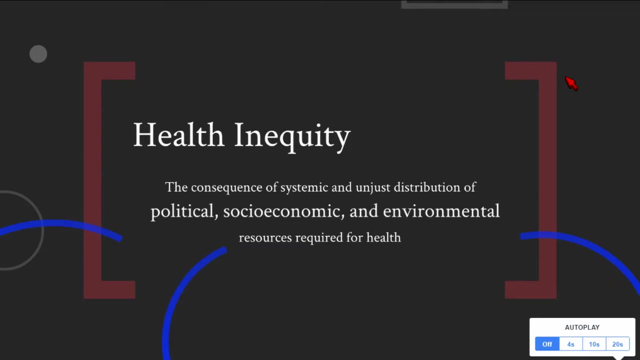 And it really brings up this question: why does being a person of color in the United States cause poorer health outcomes? Racism is a massive driver of health inequity, a concept defined by the WHO as the consequence of the unequal distribution of political, socioeconomic and environmental resources. 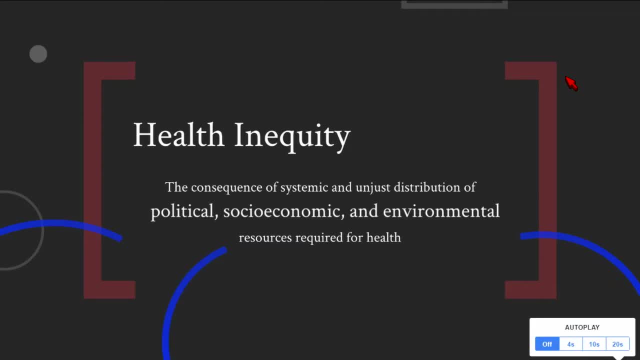 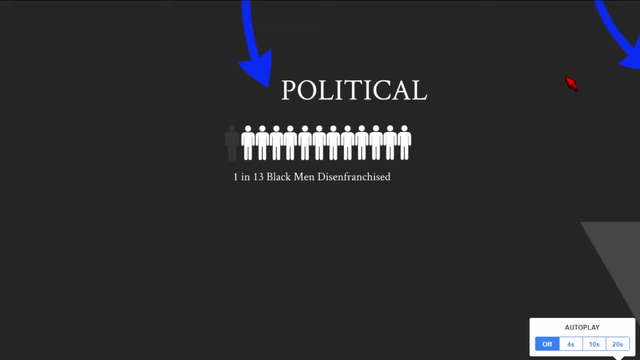 that are required for health. So consider how each of these avenues begets health inequity. One in 13 black men are disenfranchised. This is directly related to the fact that, despite similar rates of drug use, black men are 12 times more likely to be arrested for drug offenses compared to whites. 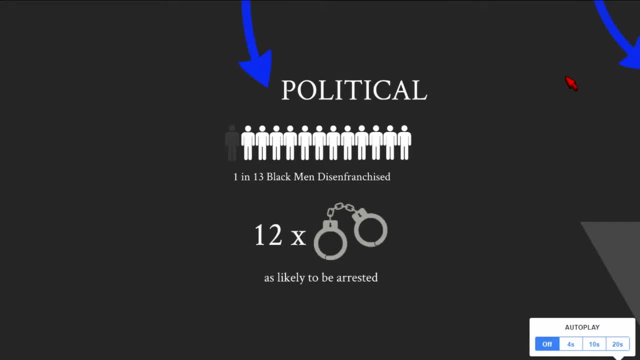 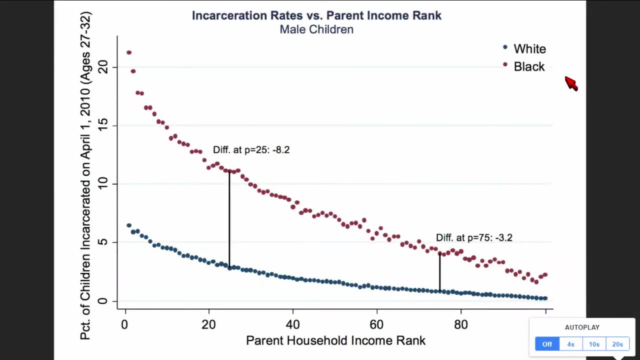 Recent data from Chetty et al at the Equality of Opportunity Project shows us that at any given time, more than 20% of black boys in the lowest income rank are incarcerated. I do not think we should be able to look at this chart without being emotionally affected. 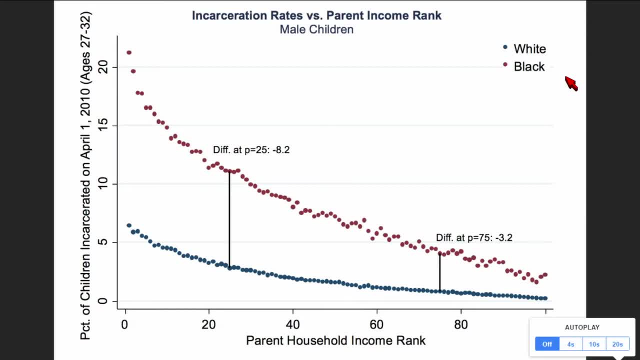 At any moment, one of five black boys in the lowest income rank in our country live in a cage. In 2016,, I was a co-teacher for a course on prisoner health and advocacy at Blackstone Academy Charter School in Pawtucket, Rhode Island. 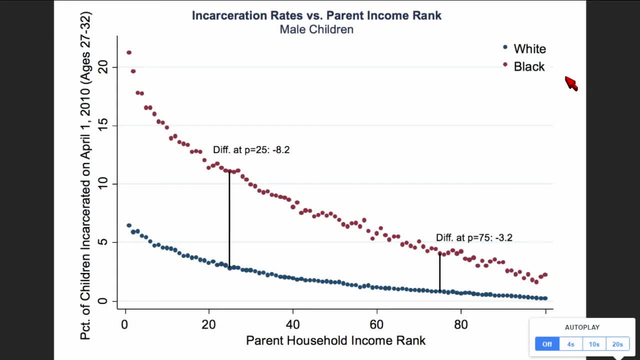 In one session we projected onto the screen the statistic that one in three black men born before 1999 will go to prison in their lifetime. At the end of my class a student touched my elbow, He pushed up his glasses and he said: 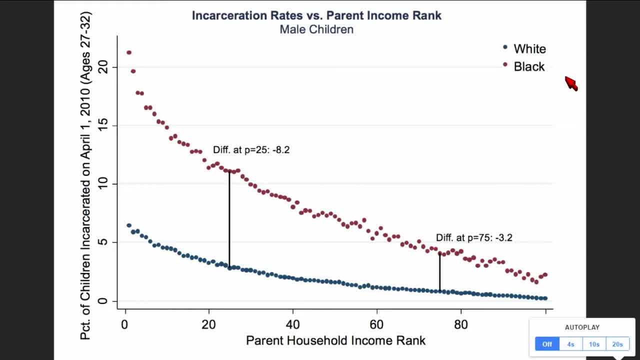 Miss Jenny. I was born in 2002.. Does that mean I will be okay? He was arrested in 2018.. So now when I go back to Pawtucket and I visit that school, I see him go to class with an ankle monitor. 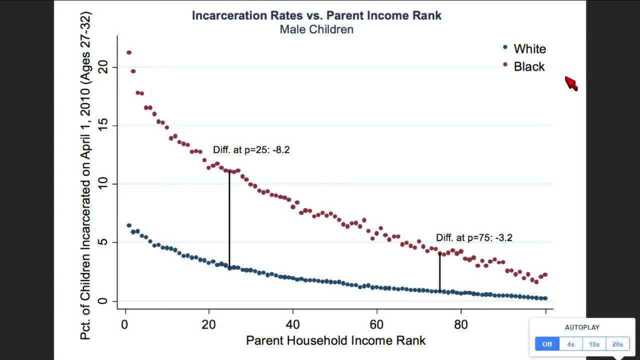 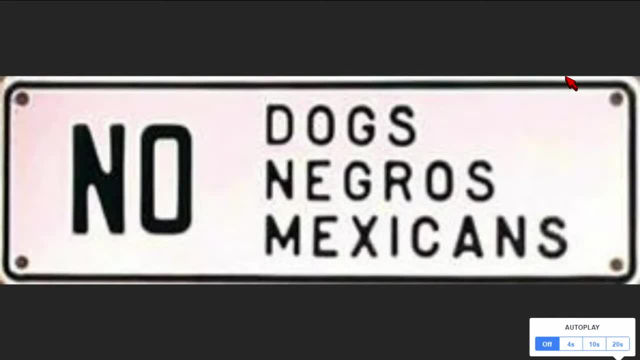 This picture represents an overwhelming amount of suffering In parts of the South. mass incarceration has rendered rates of disenfranchisement that surpass Jim Crow era levels. This serves as a potent mechanism for limiting the ability of black communities to advocate for their needs. 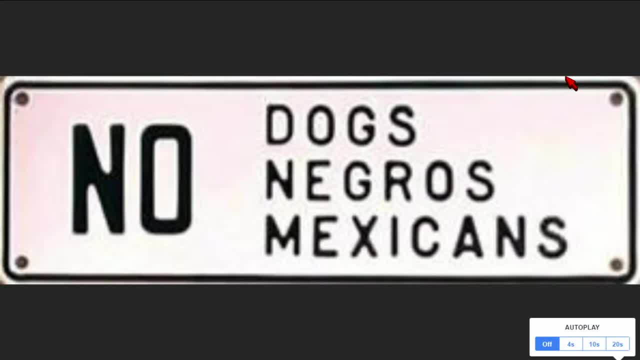 And in fact the US now imprisons a larger percentage of its black population than South Africa did during apartheid? How do we understand state violence to be a part of healthcare inequity, especially given the fact that in some regions of our country, 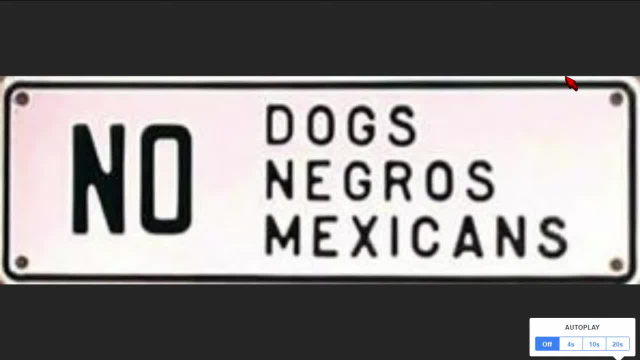 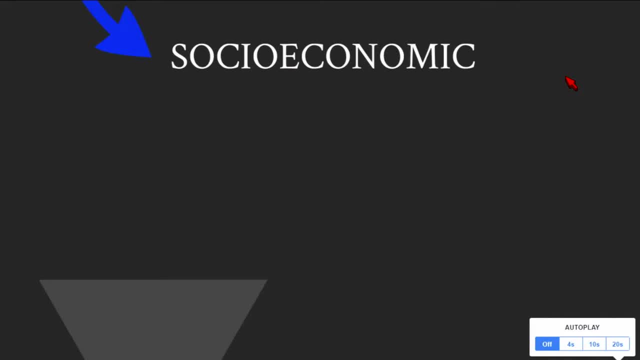 a prisoner will die every seven days due to inadequate medical care. On a socioeconomic level, healthcare access in this country is heavily dependent on what you can afford. So while recent statistics show that the median black-white income gap itself is large- 60,000 compared to 35,000 for blacks, 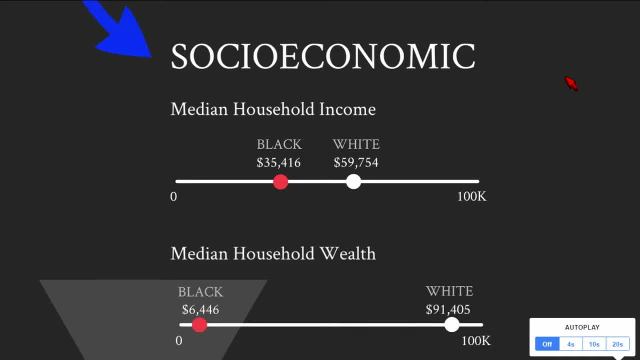 the median wealth gap is startling at 91,000 for whites and 6,500 for blacks. The median wealth of white households is almost 14 times that of black households, and this gap is widening. According to a report from 2010,, the median wealth for a single white woman was $41,500. 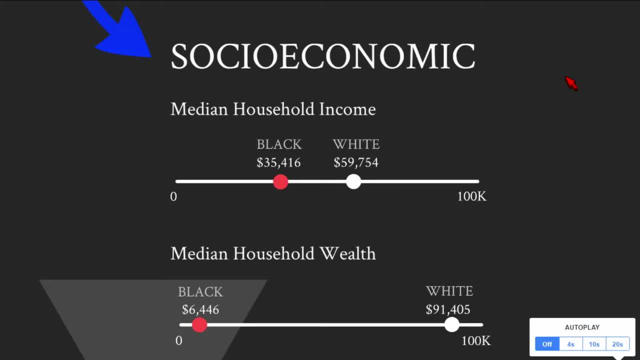 The median wealth for a single black woman is $100.. If we consider economic analysis, that nearly 50% of the median homeless population comes from the value of their property, we have to go back and analyze how black families were denied home-owning opportunities. 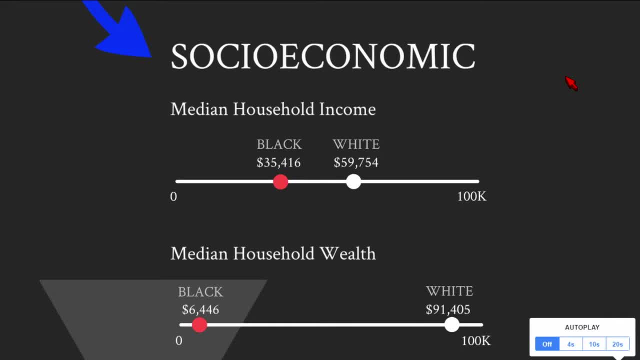 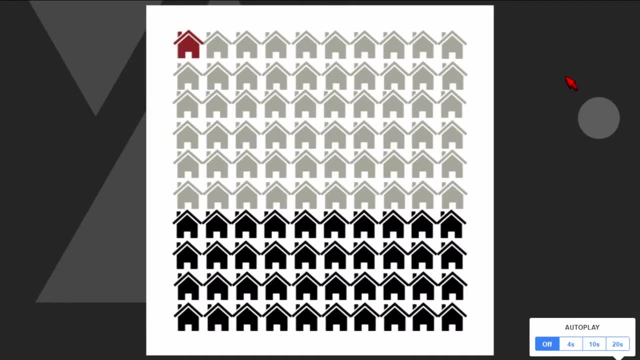 under discriminatory policies from the New Deal era. In the 1930s, the Federal Housing Association financed 60% of all American homes, yet less than 2% of these loans went to people of color. Black neighborhoods were routinely redlined and coded for mortgage defaults. 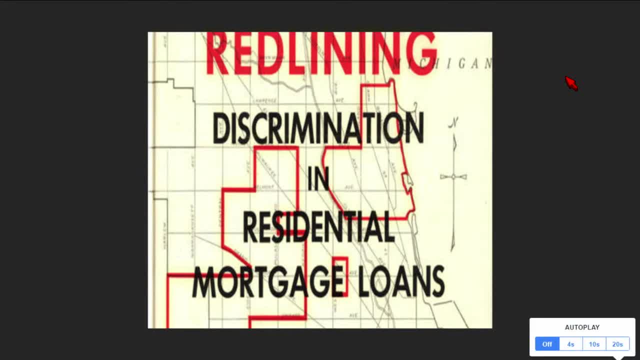 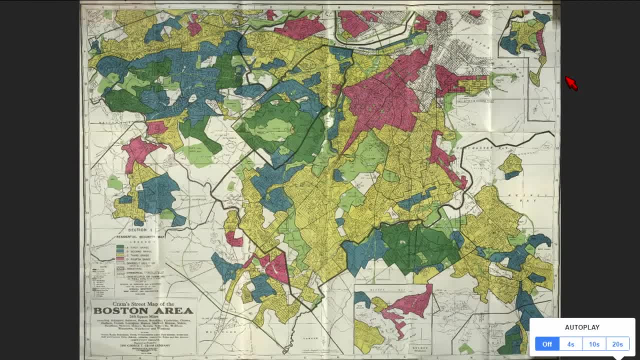 straining black families in poorly resourced neighborhoods without means for migration. This is an archival map of Boston. by the coding of the time, green was valued as best, blue still desirable, yellow declining and red hazardous. This was about denying and restricting services to residents of a particular area. 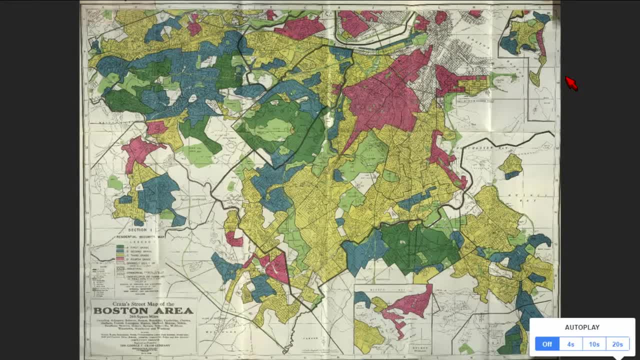 based on racial and ethnic composition, And this cordoning off of different groups of people is foundational to government-sponsored racial segregation which, even when controlled for income, is tied to low birth weight, obesity, cardiovascular disease and lower life expectancy overall. 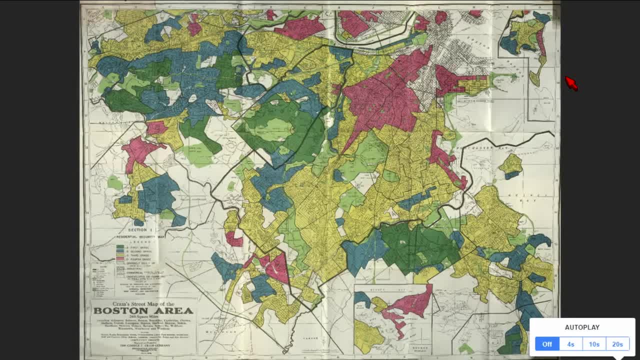 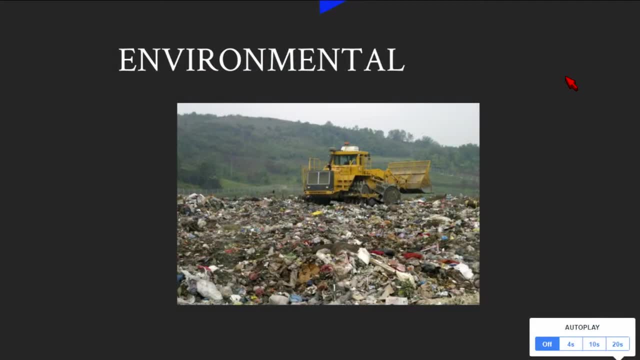 It is one of the most important factors in deciding measures of infant mortality. With regard to environment, a recent six-year study analyzing data from the Bureau of Economic Analysis, Labor Statistics and the EPA found that a significant racial gap exists between who causes air pollution and who breathes it. 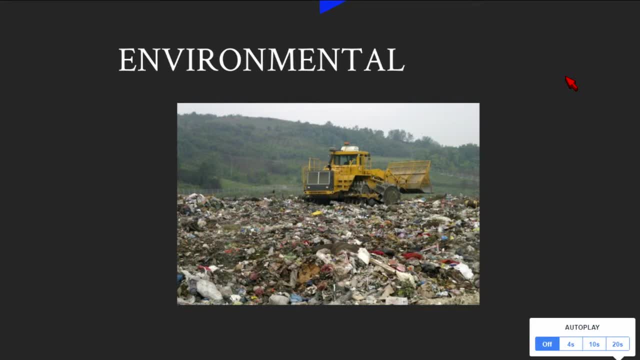 Whites experience approximately 17% less air pollution than they produce through their consumption, while black and Hispanic populations bear 56 and 63% more air pollution than they cause. People of color are continually closer to environmental health hazards like pollution and radiation, which are tied to significant increases in cancer, miscarriage, neonatal disorders and asthma. 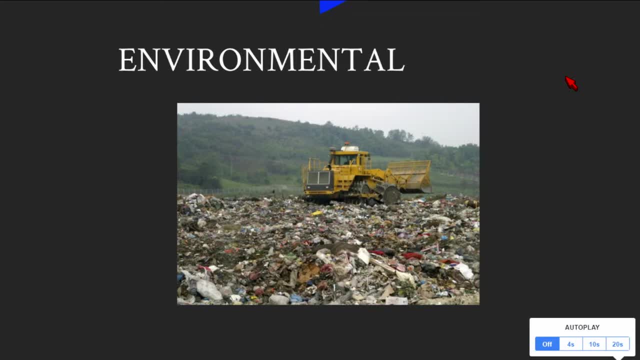 just to name a few. In fact, race, more so than socioeconomic status, is the best predictive variable in determining the placement of a toxic landfill. In sociological literature, these areas are known as fence-line communities or sacrifice zones, and to me that speaks volumes. 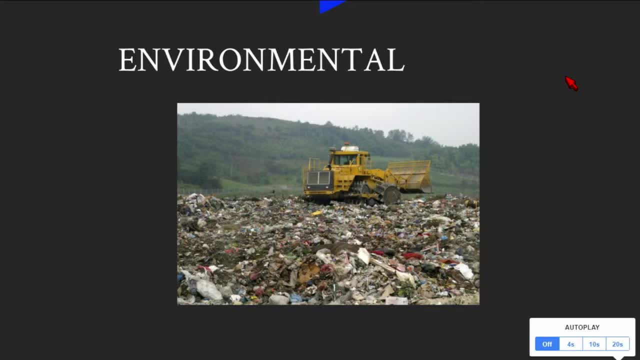 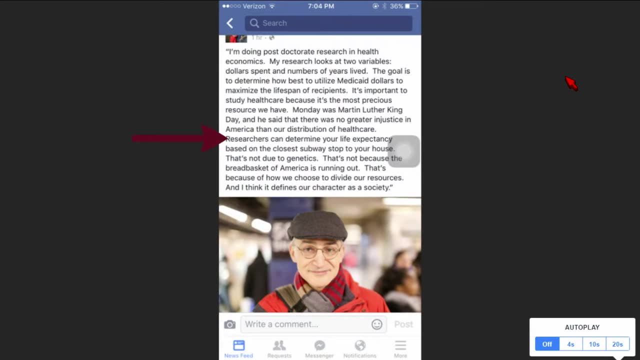 What does it mean to be an individual who grew up in a place that has already been sacrificed? I saw this on a Humans of New York post. It says Researchers can determine your life expectancy based on the closest subway stop to your house. That's not due to genetics. 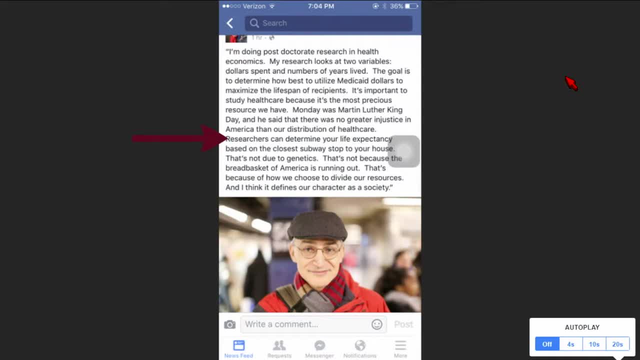 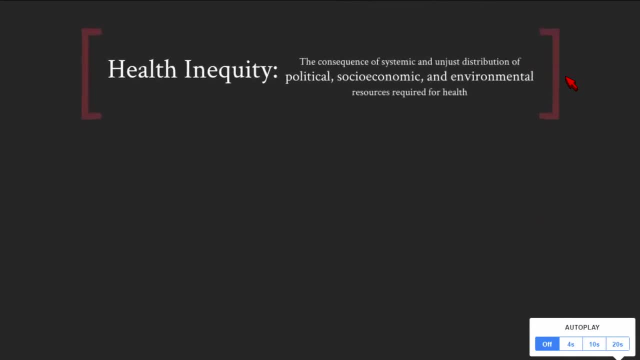 That's not because the breadbasket of America is running out. That's because of how we choose to divide our resources, and I think it defines our character as a society. The issue of health inequity revolves around central ideas of power, and these ties among mass incarceration, space, education and economic capacity are intense. 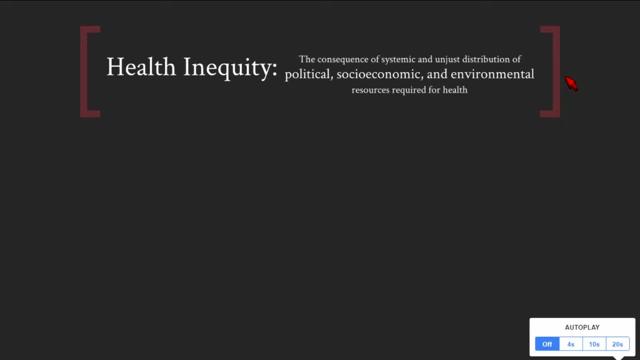 The axis of race runs through these facets and mix to create unique hostilities that build upon and with each other. Segregation exposes communities to hyper-policing, which is tied to fine farming. The Department of Justice investigated the Ferguson Police Department and found that 85% of traffic stops targeted black residents. 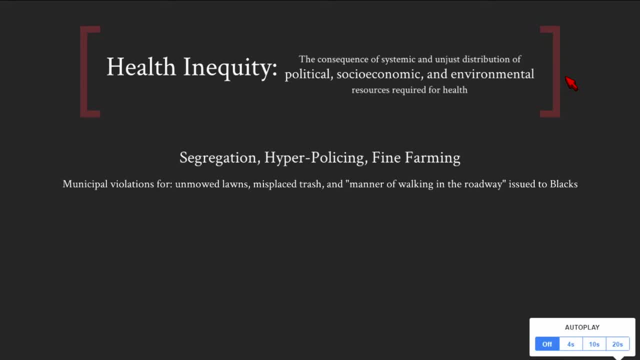 Municipal violations for having unmowed lawns or misplaced trash were issued overwhelmingly to black residents. 95% of citations for the quote manner of walking in the roadway were issued to black Americans. And what does that mean? It means money. About a quarter of African-American families in the United States have less than $5 in reserve. 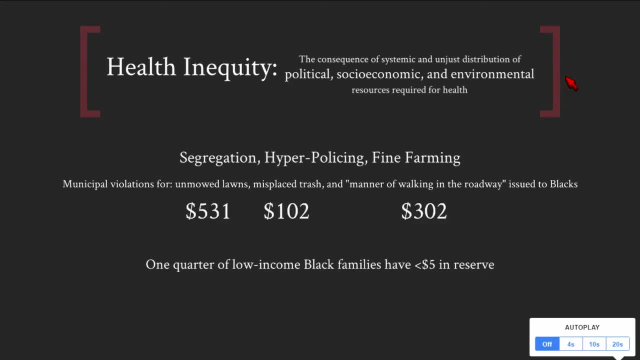 In Ferguson, the fine for high grass and weeds is $531.. $102 for misplaced trash, $302 for violating the manner of walking. And what does this mean? It means that the poorest and most vulnerable are subsidizing their municipalities. They are the ones paying for revenue gaps created by corporate tax abatements. 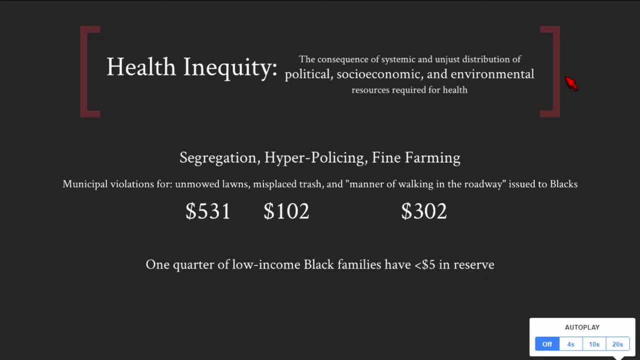 they are paying for government debts and they are being forced into predatory groups, and they are paying for loans and high-risk borrowing that we know are both financially devastating as well as racially discriminatory. We have to conceptualize racism not only as an interpersonal phenomenon. 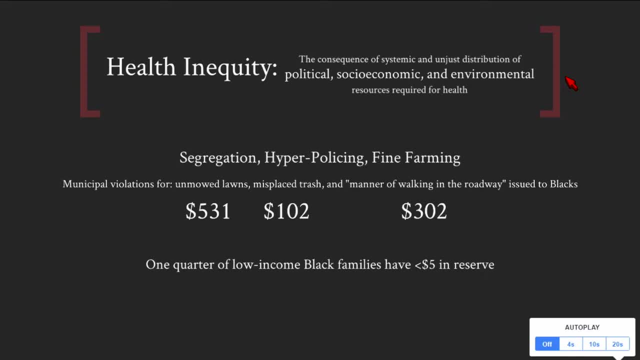 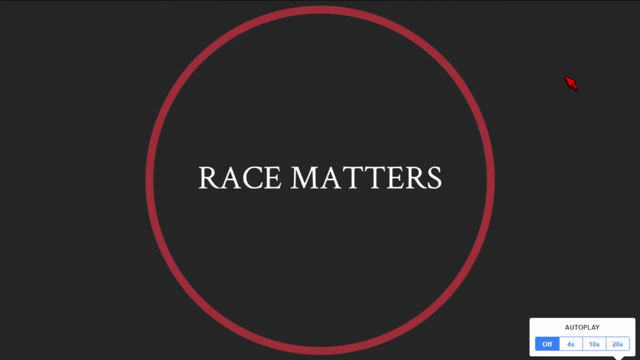 characterized by slurs and discrimination, but also as an overarching set of practices that devalue and disadvantage people of color at every and multiple levels of society. What becomes clear, then, is that race certainly matters, But what matters more is how you talk about race and how you think it matters. 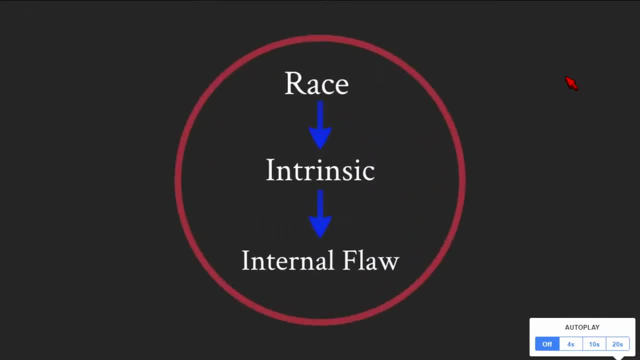 The issue here is that framing race as biologic reifies the idea that people of color are innately different, and it implies that health disparities are due to internal racial flaws only solvable through genomic technology. This diverts attention away from larger realities of social inequality. 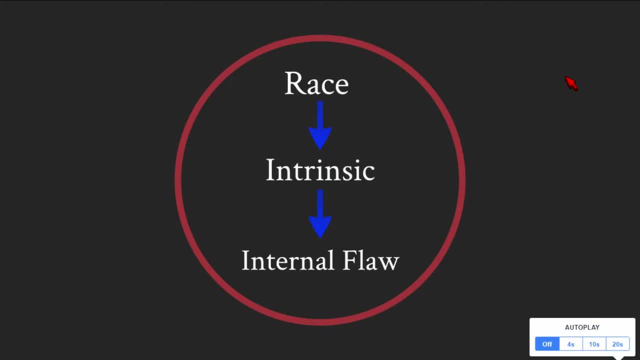 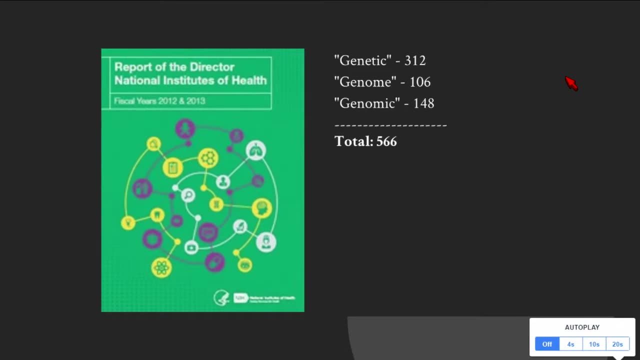 and the need for social rather than scientific interventions. In the most recent NIH biannual report to Congress, the words genome, genomic and genetic were used a total of 556 times. In comparison, a search for other words such as social determinants of health, discrimination, poverty. 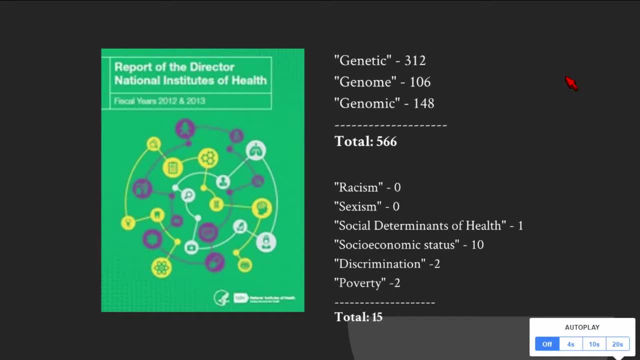 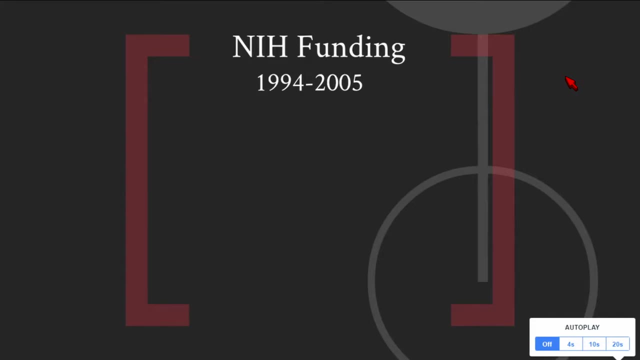 socioeconomic status. racism and sexism only came up a total of 15 times across 441 pages. If the words are not there, the attention is absent. This is incredibly important when we look at where our resources are going. From 1994 to 2005,, more than 22,000 NIH grants funded research on genetics and race. 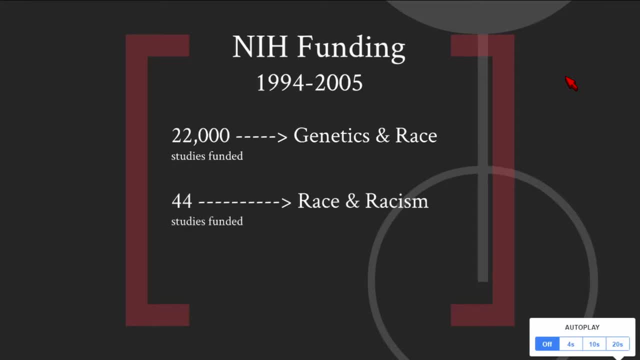 In the same decade, only 44 grants were awarded to research on racial discrimination or racism. This is a 500 to 1 ratio of spending difference that pays attention to race rather than racism, And I almost always cite this because it illustrates one of the more insidious but significant detriments of genomic research. 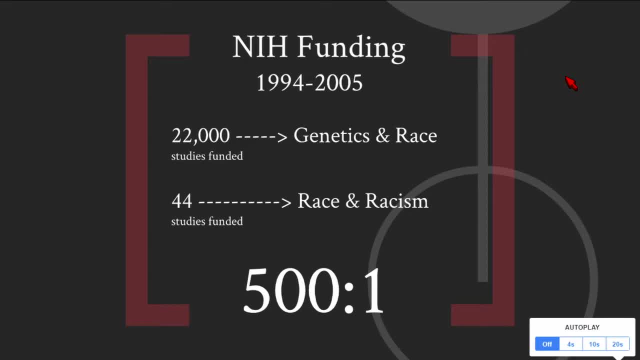 You can argue that information is very valuable, but we have to be careful to realize that mining this data is not always without cost or harm. This ties directly to issues of knowledge production and resource allocation. Recently, a $12 million grant was awarded to investigate biological 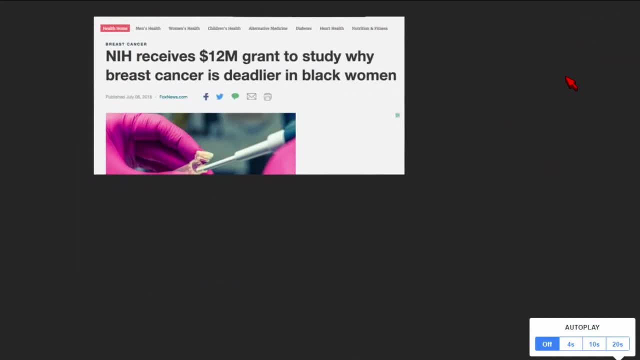 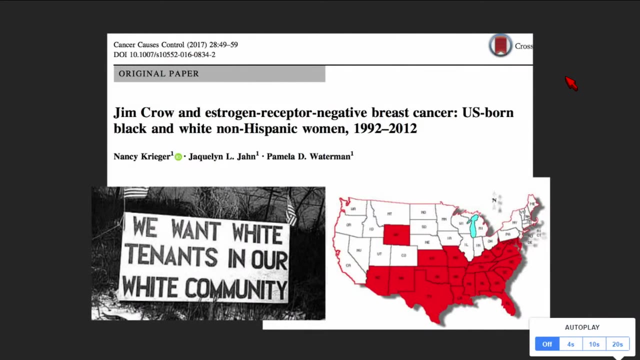 and genetic factors that contribute to breast cancer in black women. Not to say this isn't important but, as William suggests, there are many more complex issues that merit our attention as well. In fact, there's fascinating research coming out that demonstrates an increase in breast cancer in black women born in Jim Crow states. 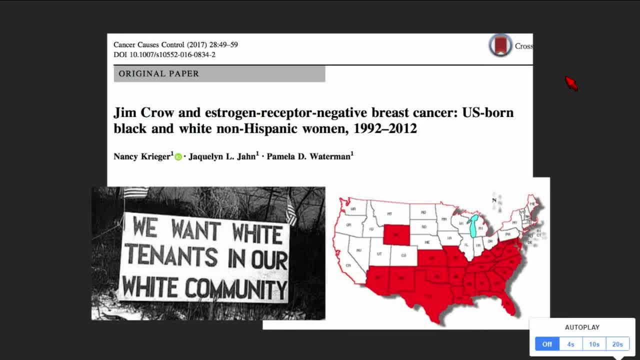 Here, Jim Crow, as a legally sanctioned infrastructure that codified discrimination has clear impacts on health and wellness, but not due to innate conceptions of race. Social context creates race-based consequences, but not due to essential biology. So how do we get studies like this funded? 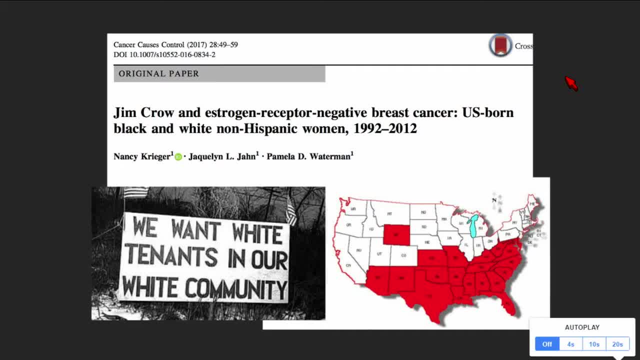 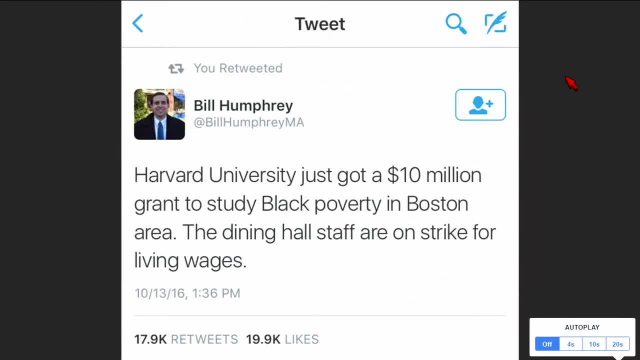 especially considering that 500 to 1 ratio. As another example, this tweet was from 2016, during union protests at Harvard. So Harvard University just got $10 million to study black poverty. in the Boston area, The dining hall staff are on strike for living wages. 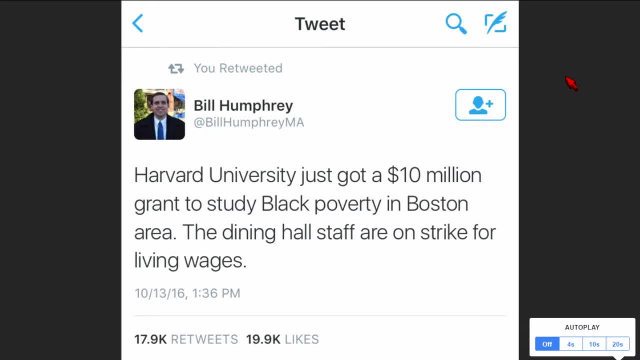 So very frequently we see these giant grants: $30 million in San Francisco recently to study homelessness- And again, that's studying. That's about this cottage industry of research and racial disparities, but the issue of homelessness has to do with housing. So why don't we spend $30 million on building houses? 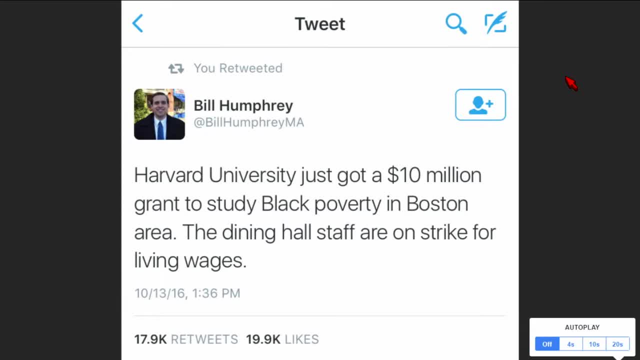 The 500 to 1 resource allocation implies that the solution to racial health care disparities lies in the investigation of racial genetics. But the next time you read a study that makes claims on clinical efficacy or health disparities based on the biology of race, question the facts that are being presented to you. 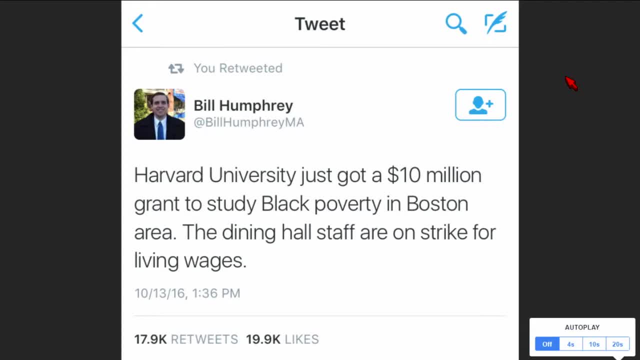 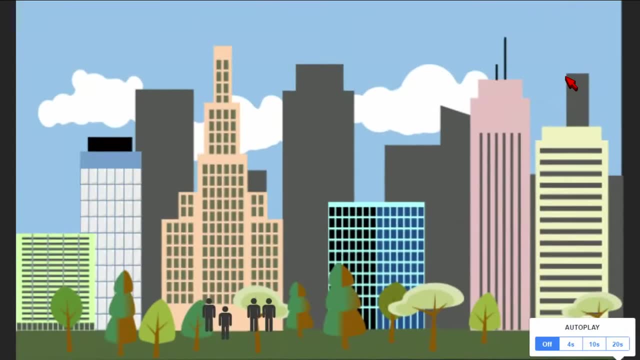 Think about how pinning health inequity on genomic difference is in the best interest of people in power and serves as a diversion from bigger issues. Systems, in addition to people, create health care disparities. but the idea of race as intrinsic not only echoes eugenic theory. 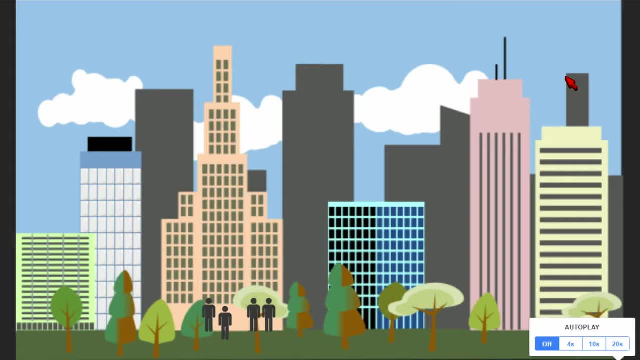 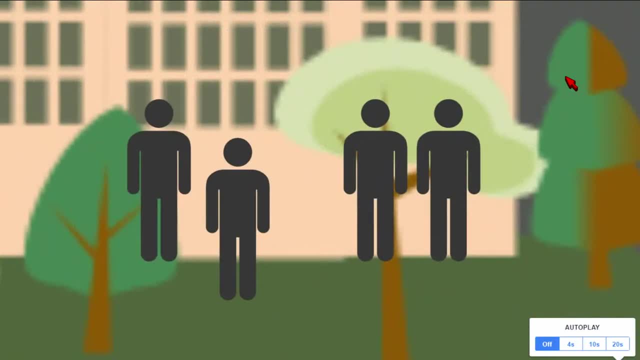 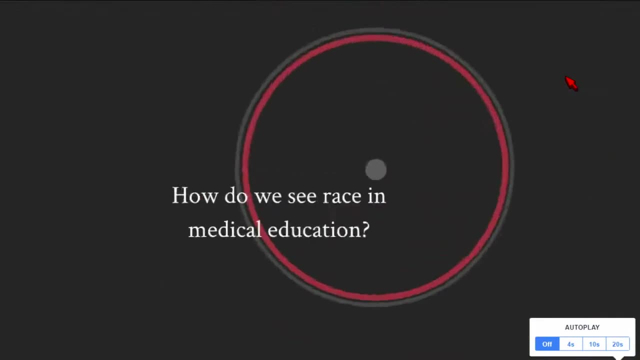 but also diverts culpability and responsibility from society down to individual people. This creates a very myopic view and it's impossible to understand the landscape. if we whittle down these massive inequities down to individual and personal genomics, The pervasive framing is heavily implicated. 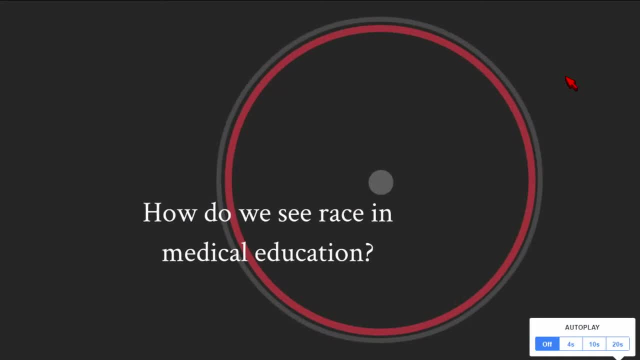 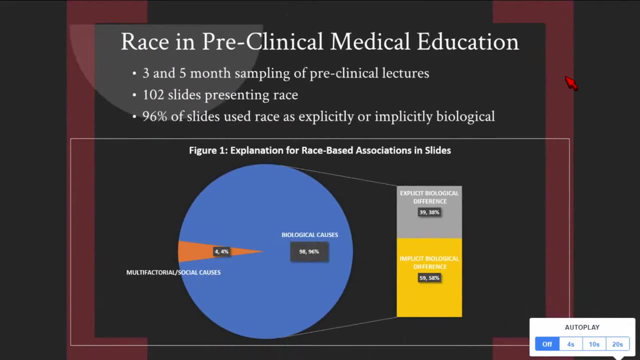 in the ways that biologic assumptions of race are operationalized and ingrained in medicine. In a three- and five-month sampling of first- and second-year preclinical curriculum at the Warren Alpert Medical School, a full 96% of lecture slides presented racial signifiers. 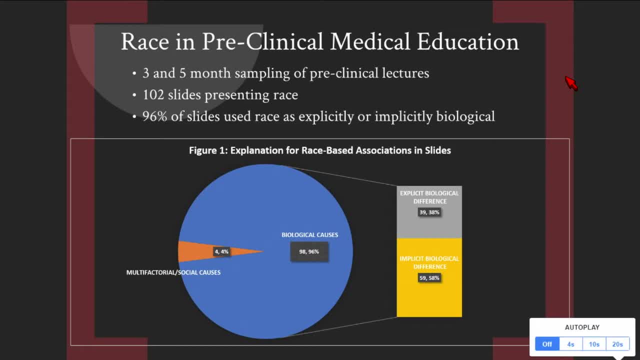 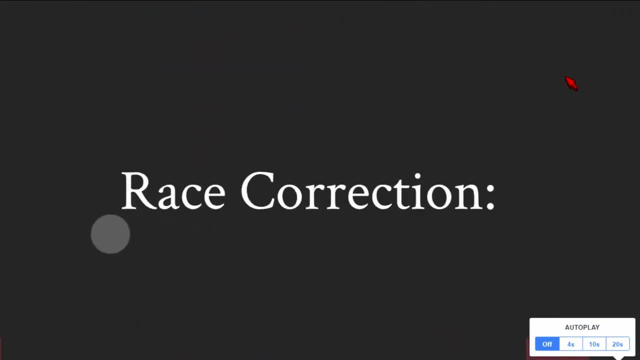 as explicitly or implicitly biologic, in association with health care disparities. For example, calculations for organ function, including lung function, measured through spirometry advocate for race correction, which is a concept that relies heavily on this idea that people are of different races. 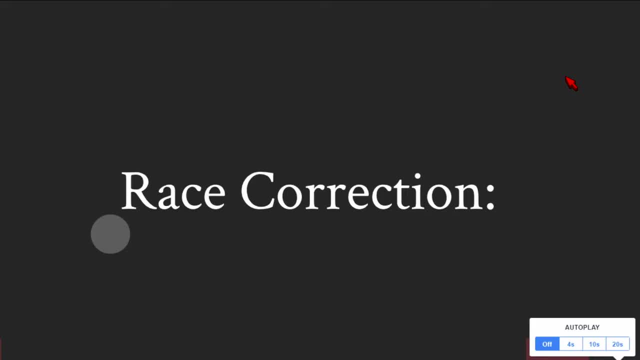 are biologically different and therefore require a correction, usually from a white standard. This concept is highly contested in scholarly disciplines outside of medicine. yet discussions of race corrections in medical education often fail to include necessary context. Spirometry, for example, is often taught. 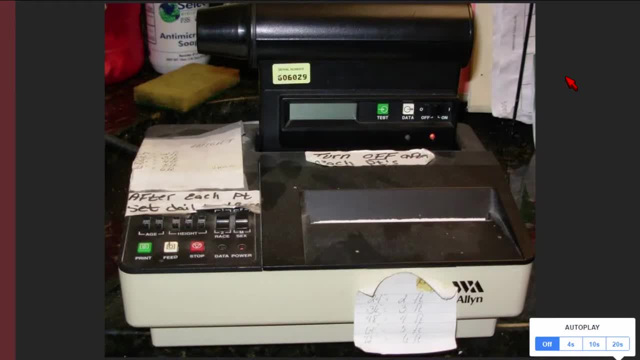 without consideration of its development, use or accuracy. despite historical underpinnings in plantation slavery, The foundation of this correction comes from efforts that were used to justify slavery. Prestigious medical journals of the time posited that lower lung function provided evidence that lack of structured labor would lead to black deviance. 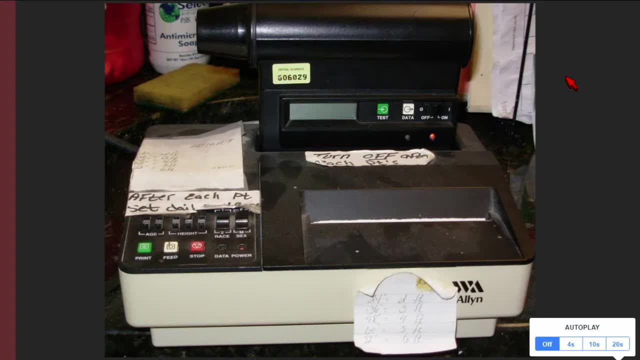 Instead, forced physical exertion was justified to keep minds free from- quote- ignorance and barbarism. In other words, the lung physiology of black people was such that slavery was integral to keeping them healthy. On this picture you can see an arrow pointing. 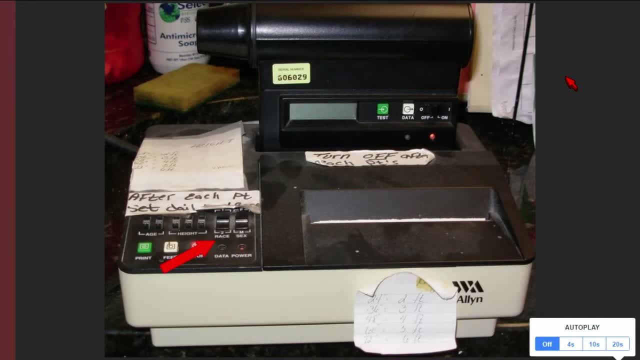 to a tab denoting race built into the machine itself so that it automatically adds this race correction to the produced report. This practice is not benign. The utilization of race correction in spirometry causes lower rates of eligibility for disability in black Americans. It essentially changes the threshold. 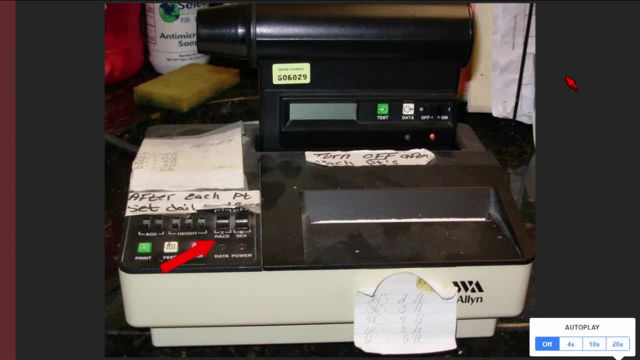 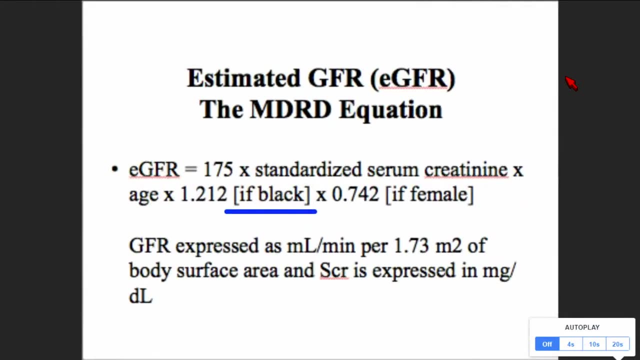 for diagnosis and disease, which has led to reduced support. GFR is another calculation that includes race as well as sex correction. In the lab, the kidney function of black patients is inflated by 20%, which is damning given the significant racial disparities. 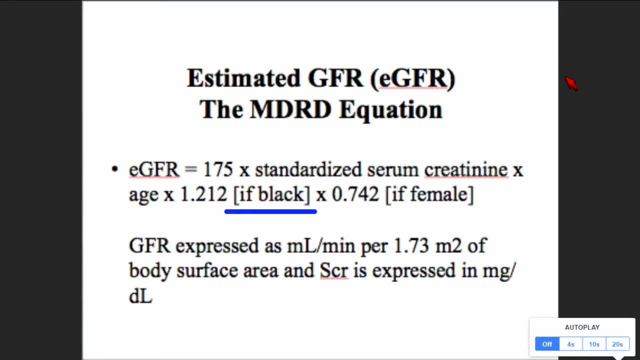 in the morbidity and mortality of kidney disease. So GFR is one of the main metrics used in deciding transplant decisions. Time on the wait list is accrued by demonstrating disease severity. Inflated function means that black patients don't get put on the list until it is too late. 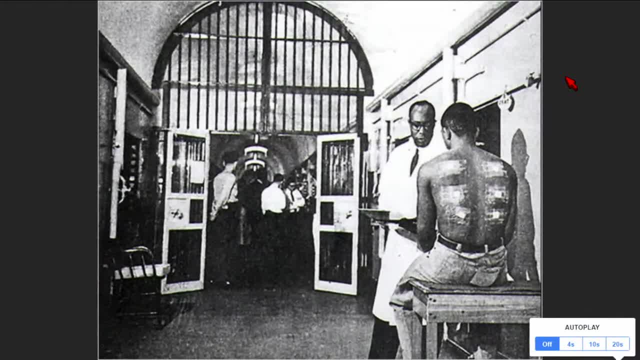 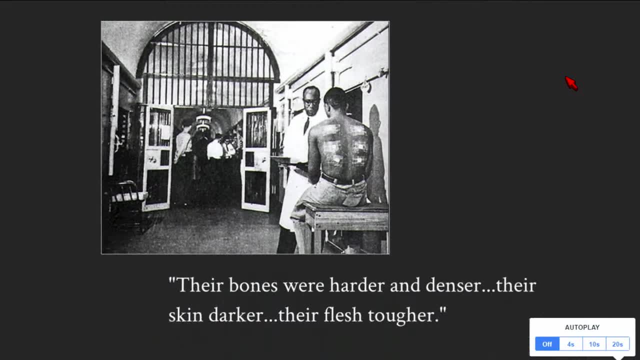 And as a historical example. for decades, doctors and x-ray technicians were taught and believed that radiation doses for African Americans should be increased because their bones were harder and denser, their skin darker, their flesh tougher. This practice caused an innumerable amount. 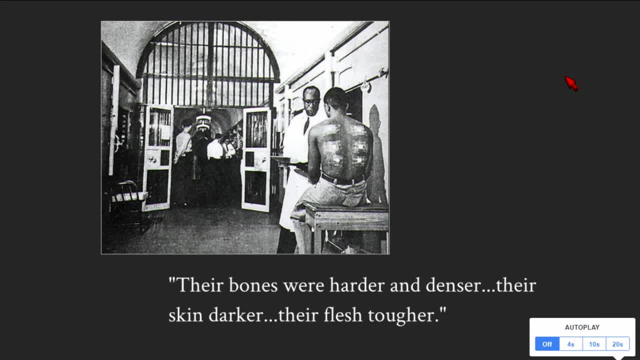 of disease and damage, and included a series of radiation experiments conducted on unknowing black patients in order to develop radiologic technologies. This practice, however, was not explicitly outlawed by the New York State Health Department until the 1970s. And in case you believe this kind of thinking, 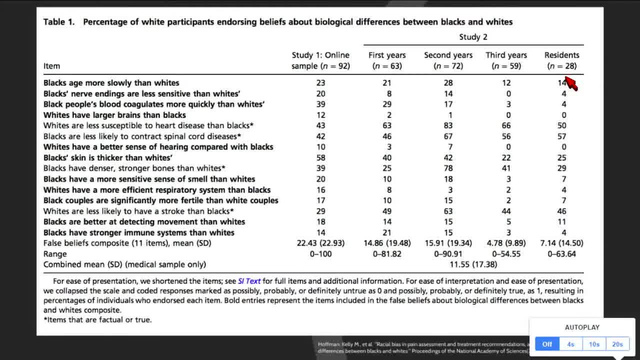 is a historical artifact. a study from the University of Virginia published in April of 2016 indicates that a significant increase in the number of medical students and residents still believe in fundamental biologic differences between whites and blacks, including that their nerve endings are less sensitive. 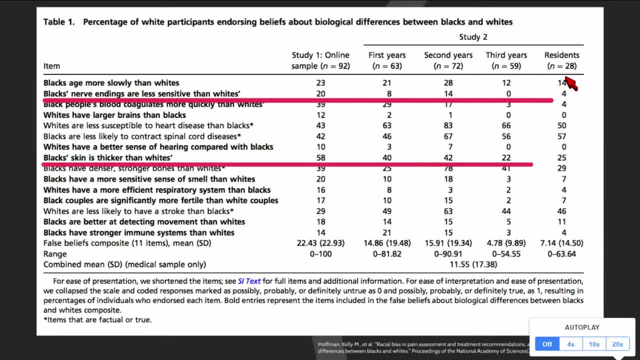 black skin is thicker and, again referring back to spirometry, that whites have a more efficient respiratory system than blacks. This is not ancient history. These ideas persist and pervade today. I think a lot of people look at eugenics and say, oh, that was like quack science. 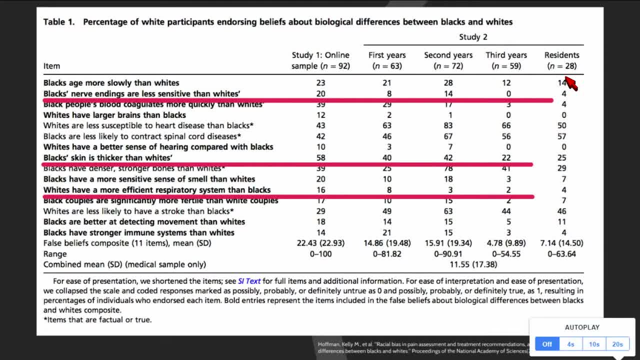 those you know were pseudoscientists that don't have anything to do with doctoring today, But this legacy is extremely important and extremely elite and well-educated. Looking at the history of Harvard, it was a huge center of eugenic thinking. 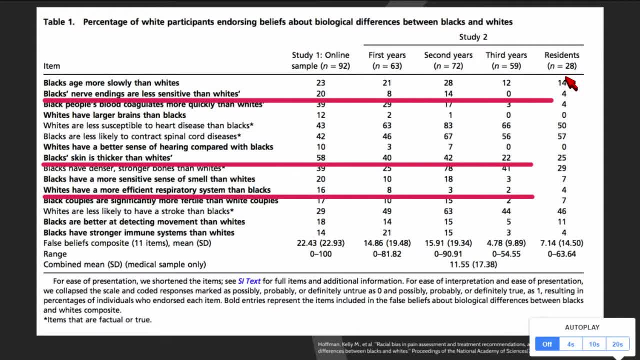 By the 1920s it offered 336 courses on eugenics as a quote, staple of biologic curricula. This is included by work, included work by former medical school deans and presidents. These ideas were considered fundamental to physician training not that long ago. 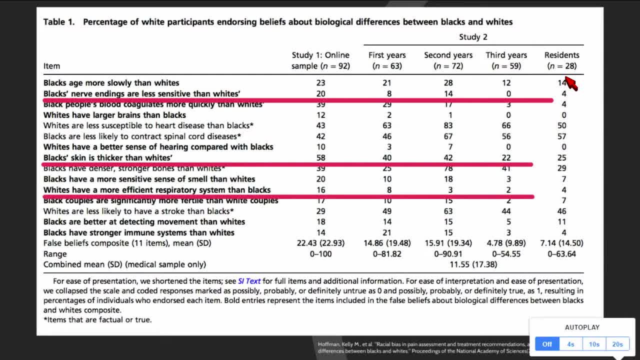 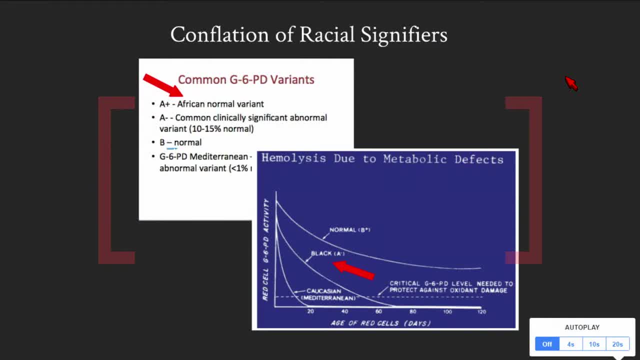 and in fact rewarded, when you think about how those careers were made. In this study, one lecturer from medical school discusses the same concept of hemolytic anemia but conflates black and African as racial signifiers. So black refers only to black skin phenotype. 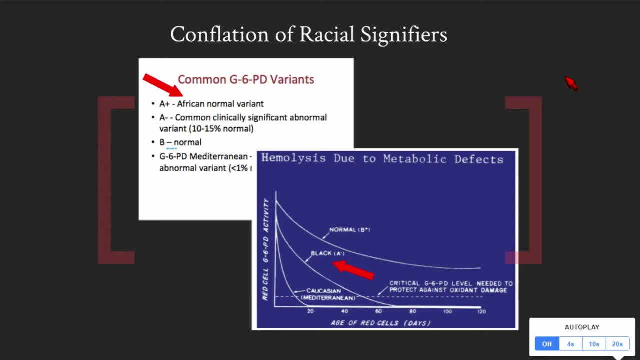 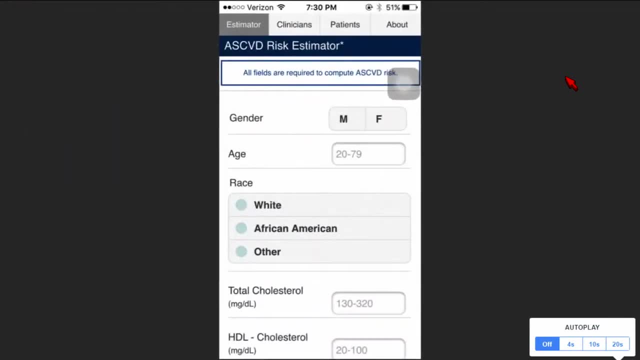 which includes all nationalities and upbringings, as well as geographic origins from sub-Saharan Africa, the Afro-Caribbean, Middle East and Latin America. Tools like the ASCVD risk calculator ask if the patient is white, African American or other. 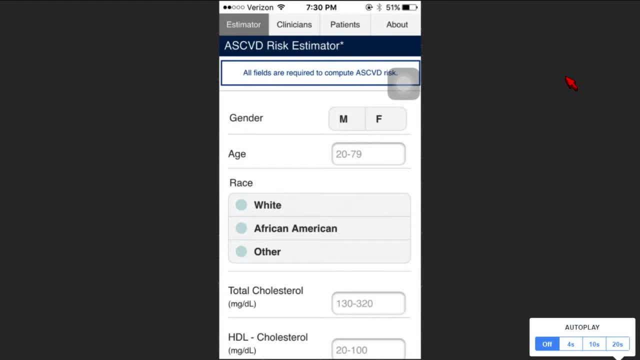 but is the African same as black, the same as African American, the same as Nigerian? How much does it matter if they've immigrated recently, not so recently? In academic and clinical medicine, we rarely know what we're talking about when we mobilize labels of race. 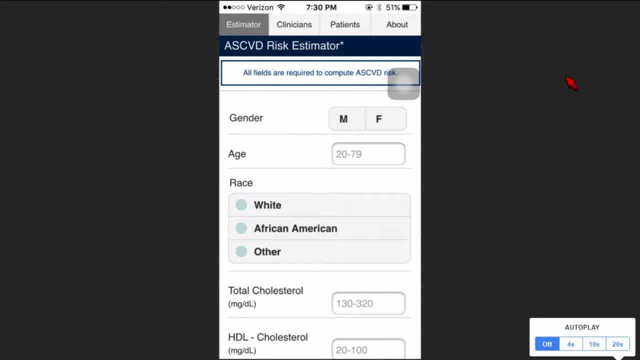 A review of NIH genetics research between 2001 and 2004 found that zero manuscripts defined their use of race or ethnicity. Not a single author articulated what they meant or how they understood race, even as they studied it. To me, this speaks clearly. 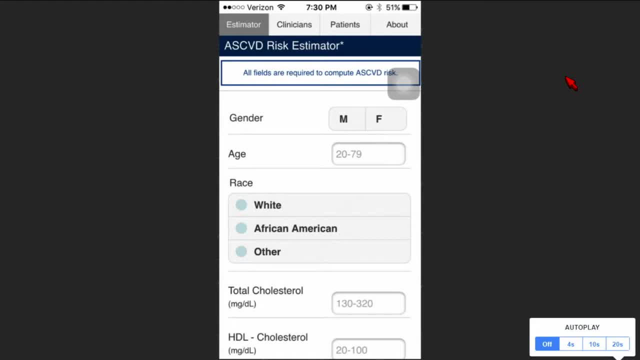 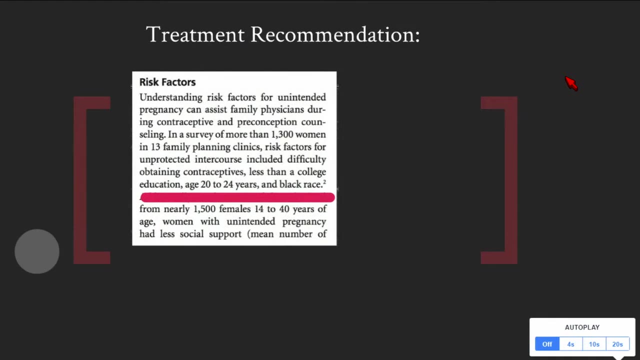 to how normalized and unquestioned biologic racial difference has become to biomedicine. In this context, can a scientific paper fail to define a major research variable? In multiple education materials from medical school, race has been listed as a risk factor for a variety of pathologies. 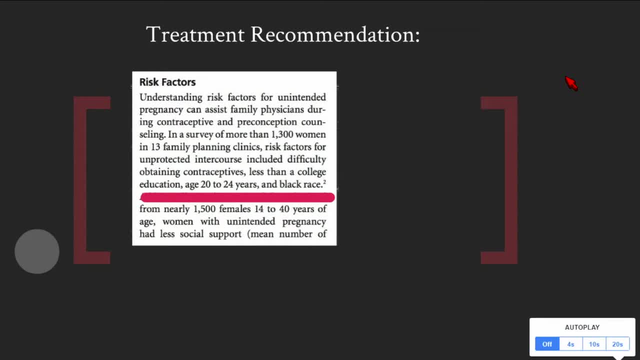 including pregnancy and STIs. So this is from the AAFP and students are told risk factors for unprotected intercourse in this pregnancy include difficulty obtaining contraceptives, less than a college education, age 20 to 24 years and black race. 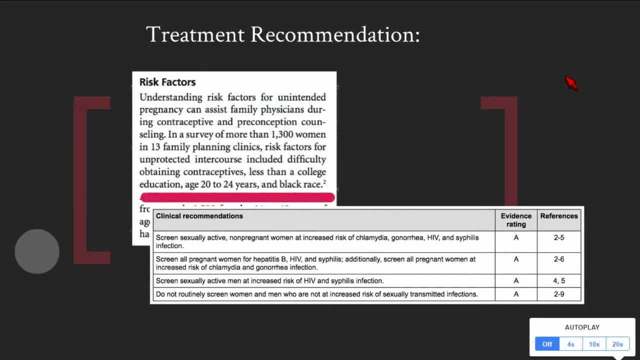 The next picture is a screenshot from the USPSTF. a different clinical practice depending on those risk factors, with no further explanation. So being viewed as black is in itself enough to qualify you as at risk for STIs, meaning doctors should routinely do STI testing. 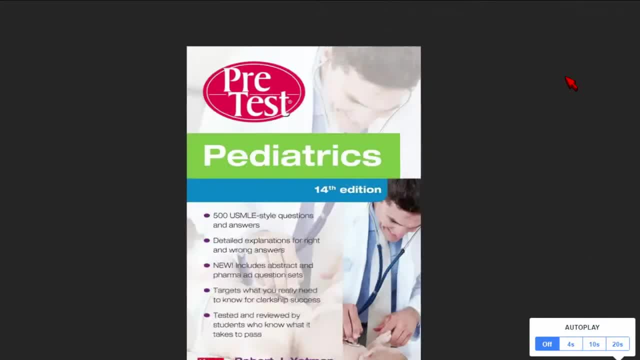 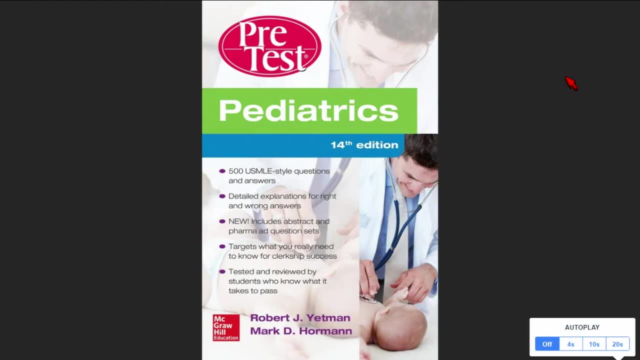 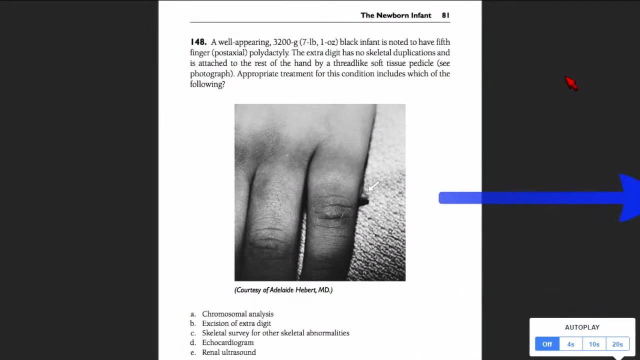 when they otherwise would not. Found another example of race-based medicine in pretest pediatrics, which is recommended as a resource for medical students. unless you went to Yale, they don't take shelf exams, which I am also bitter about. A well-appearing black infant is noted to have. 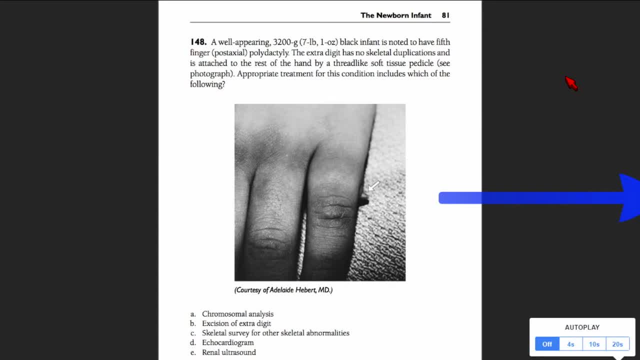 post-axial polydactyly. The extra digit has no skeletal duplications and is attached to the rest of the hand by a thread-like pedicle. What is the appropriate treatment? You can choose chromosome analysis, excision, skeletal survey, echo or ultrasound. 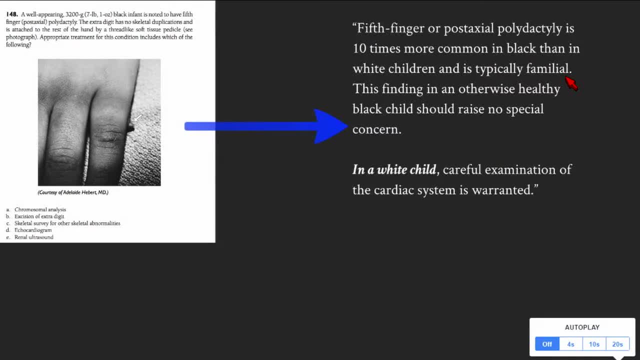 The answer states: fifth finger or post-axial polydactyly is ten times more common in black than in white children and is typically familial. This finding in an otherwise healthy black child should raise no special concern In a white child. careful examination. 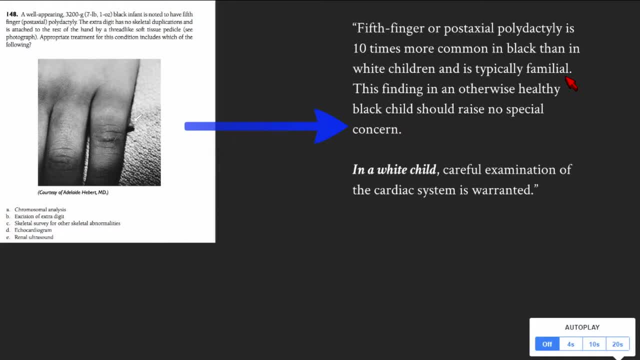 is warranted. It goes on to note some syndromes that are associated with this polydactyly, and they include Rubenstein-Taby syndrome, Mecklen-Gruber syndrome and Ellis-Van Craveld syndrome, the consequences of which include. 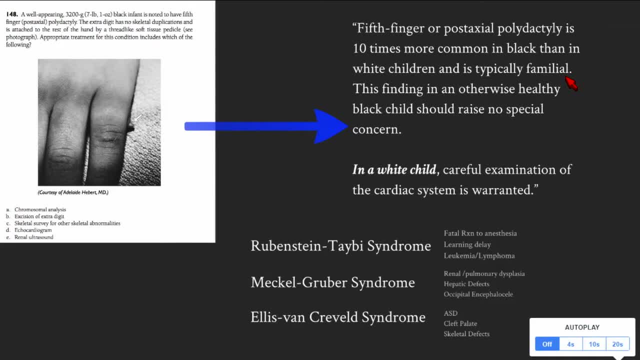 fatal reactions to anesthesia: leukemia, lymphoma, kidney, liver and lung dysplasias, atrial septal defects and dwarfism. So these are very serious complications to be gambling with with the heuristic of black, white, otherwise healthy. 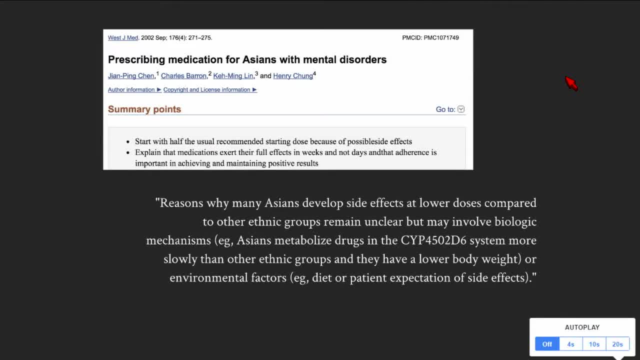 In addition to this, there are other factors associated with lower initial doses of antipsychotics due to increased side effects. The authors of this review themselves postulate that this may be due to genetics, lower body mass, diet or patient expectations of side effects. 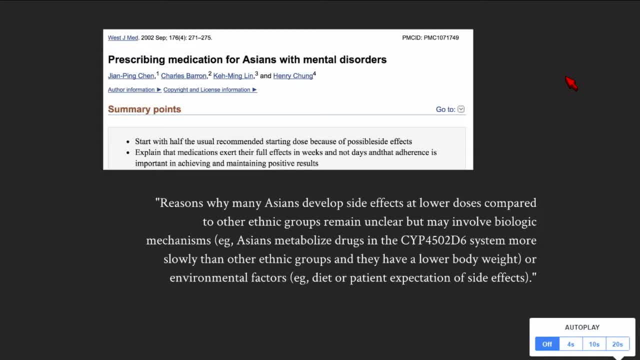 When race is used as proxy in this way. it's not thoughtful, It's sloppy. Asian is not a representation for all of these factors. We've seen data that this kind of study was used in the clinical office If it's about expectations or diet. 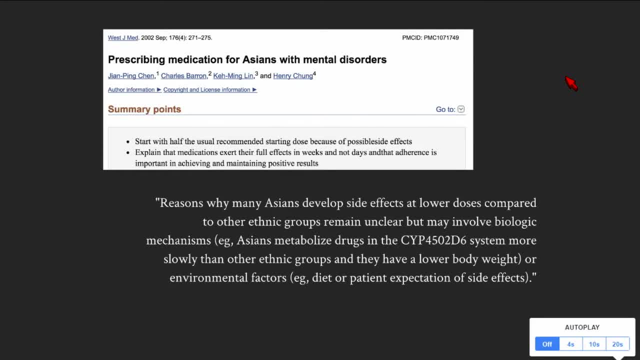 we can assess those directly. A 1991 study published in JAMA suggested that AZT had no benefit in HIV-positive Latino men. It was later disproven under questions that lack of control for socioeconomic status, access to health care and higher disease severity at presentation. 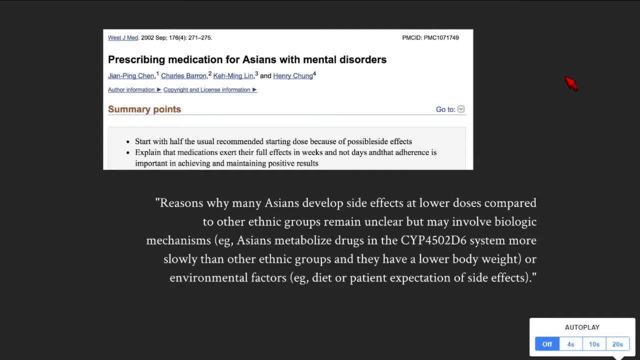 confounded the results. And yet the study influenced medical management. Doctors withheld AZT from Latino men with HIV under the assumption that it was not efficacious for their assumed racialized biology. I want to touch very quickly on racialized health disparities as a bit of a case study. 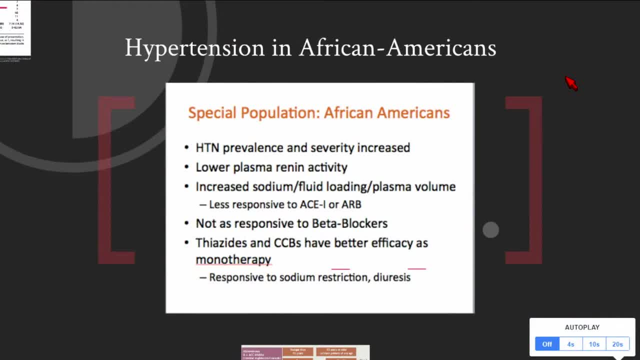 but it can't really cover the current literature. There's a lot out there, But this is a lecture slide from our second year, where, as students, we are taught that African Americans are less responsive to ACE inhibitors and should be put on other medications first. 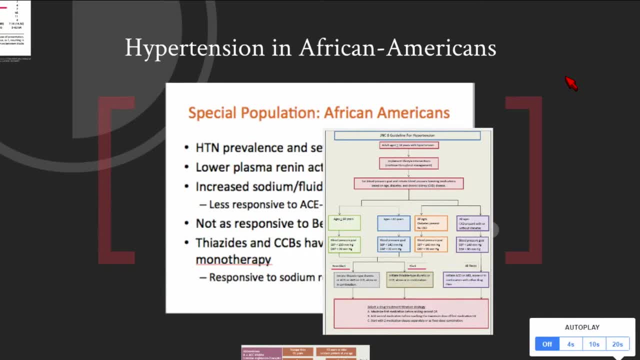 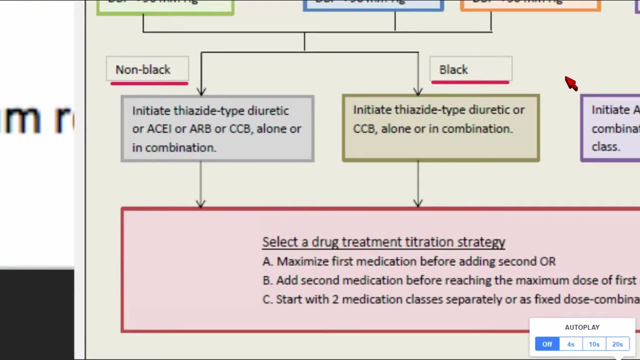 And indeed this follows the hypertension guidelines from the JNC-8, which includes an algorithm that directly separates treatment recommendations from the JNC-8.. Interestingly, guides in the United Kingdom mirror the JNC-8, except they have one difference. 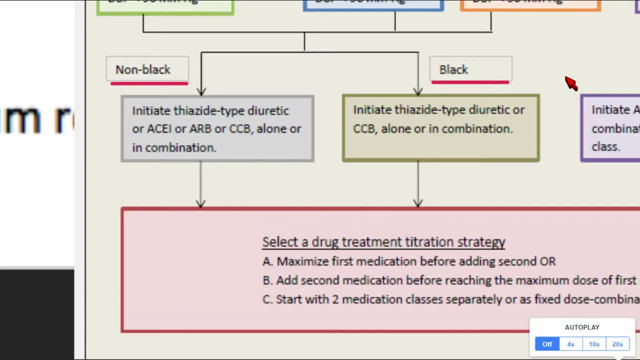 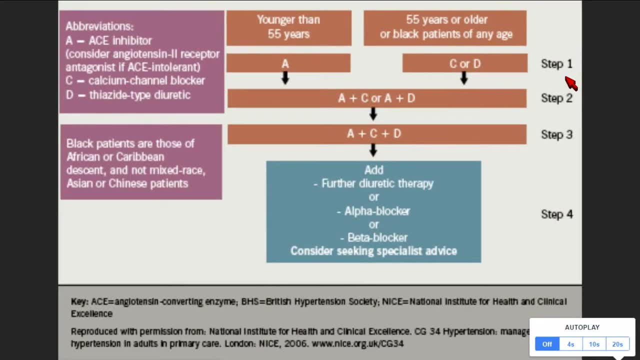 They explicitly direct that guidelines for mixed race do not differ for those recommended for whites, Asians or Chinese. So first, again, it shows this fact that across borders, racial labels mean something very different In my mind. China is in Asia. 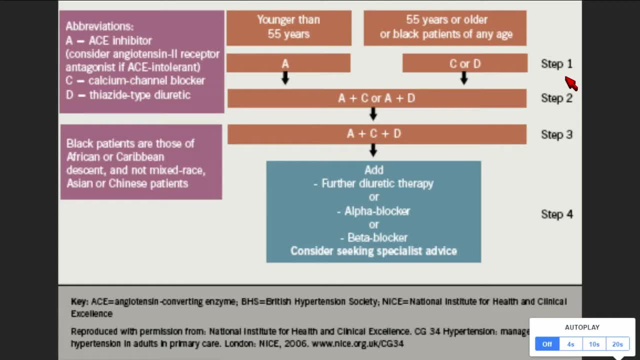 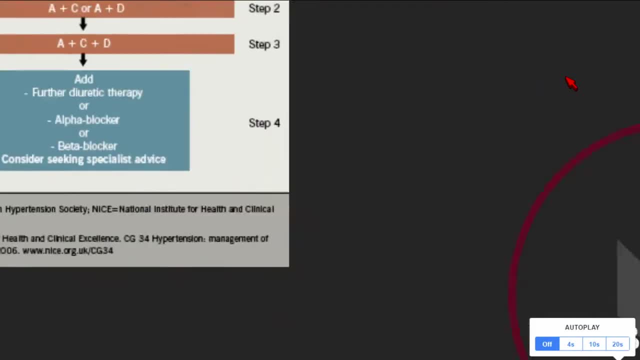 so Chinese are also Asian, But it means something really different across the pond. And again it's an example of we don't know what we're talking about when we use these things. This also brings up Plessy's question from 1896.. 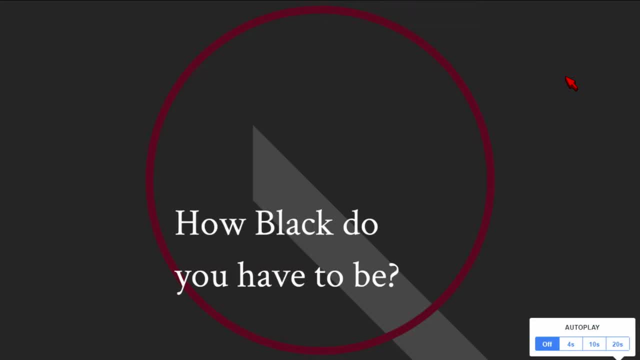 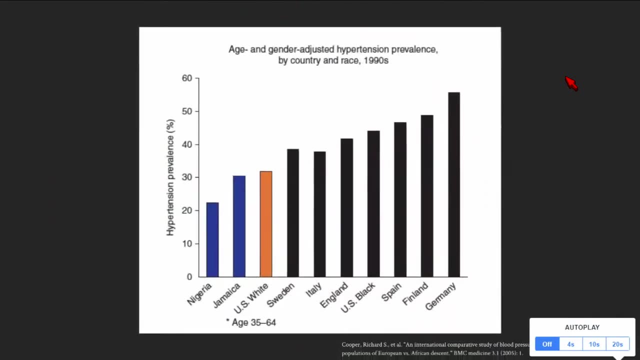 How black do you have to be to be black enough? This time, instead of asking the courts, we're asking physicians to provide the answer. Internationally, African Americans suffer hypertension at rates 3.5 times those of Nigerians living in Africa. 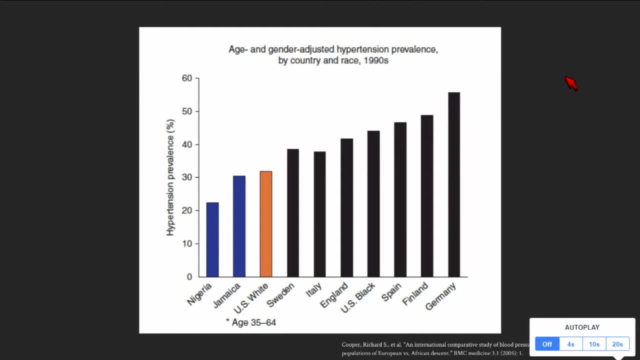 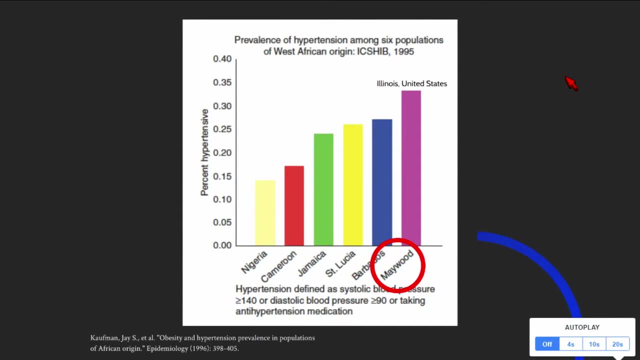 African Americans experience hypertension only 0.7 times the rates of presumably white Germans in Germany. From another study, rates of hypertension in black individuals from Illinois are shown here, compared to five countries of West African origin. If you truly believe that there is something, 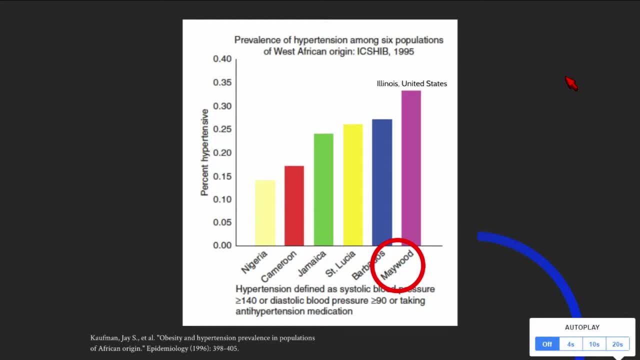 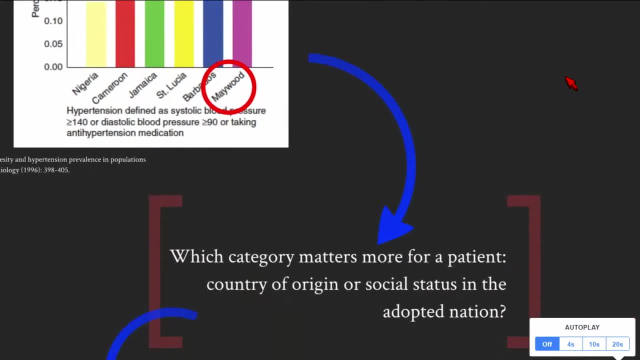 about the genetics of African populations that predispose them to hypertension. it's really difficult to explain these results. Instead, it poses a different question: Which category matters more for a patient: Country of origin or social status in the adopted nation? It seems that there is something about the US. 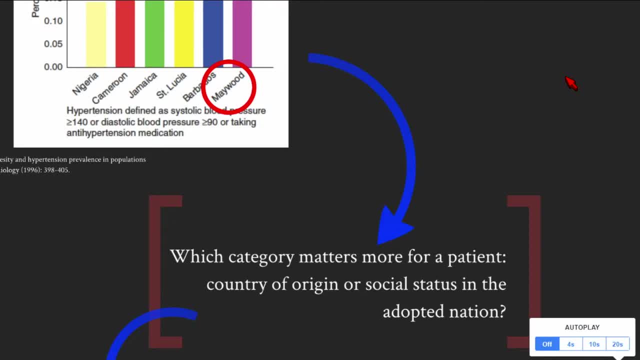 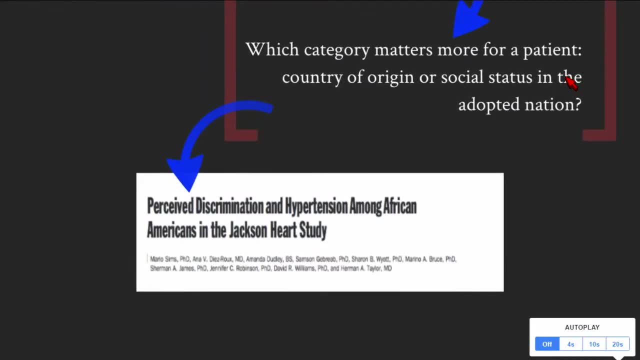 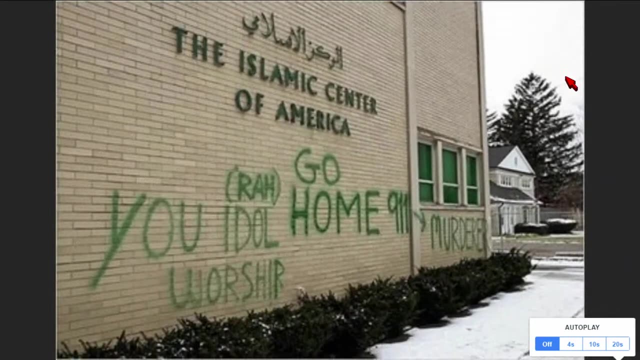 not African genetics or ancestry that is the source of hypertension disparities in America. In fact, research from 2012 began exploring correlations between metrics of discrimination with rates of hypertension In California. women with Arabic names who were pregnant in September of 2001. 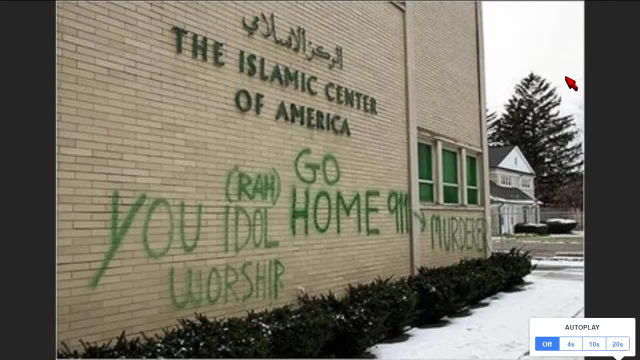 and the aftermath of 9-11 had significantly higher incidence of low birth weight compared to similar populations who gave birth a year earlier, in September of 2010.. This incidence correlated with a three-fold rise in Middle Eastern hate crime in California and demonstrates that race stress 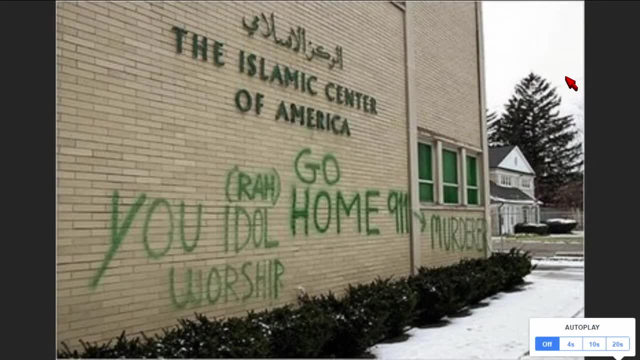 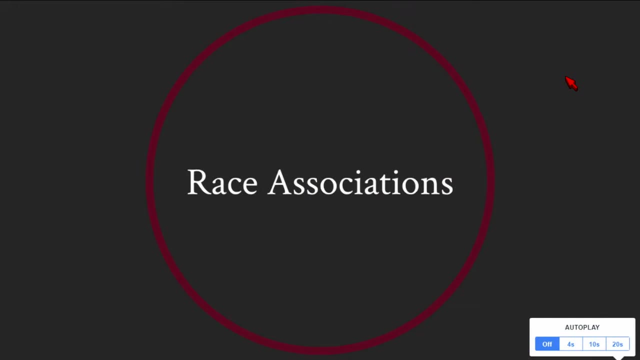 and health are still intertwined. Additionally, and this is more relevant to the doctors in the room, inaccurate biologic concepts of race without critical examination have negative clinical consequences. So I would argue that, due to board examinations, every US medical student of this generation is aptly familiar. 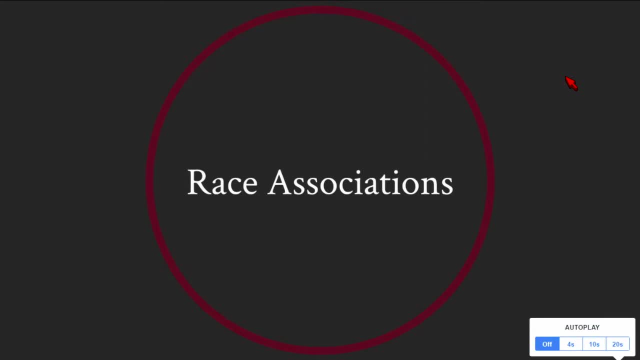 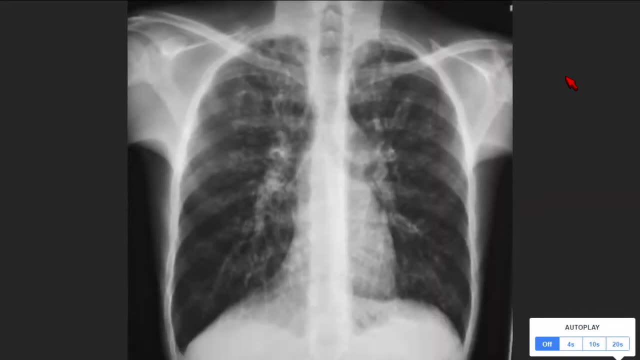 with race associations. Yet repeated ideas in this way can result in misdiagnoses or delayed treatment. if patients present outside of the structured period die, There's a case study in which a young African American girl is in and out of the hospital for years. 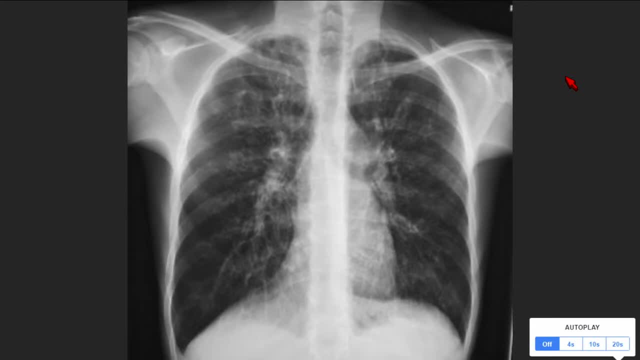 looking for an answer for her recurrent illness, And it's not until a passing doctor sees her x-ray and asks who's the kid with cystic fibrosis that she gets her answer. Because of the way CF is so often associated with white children, this patient lost. 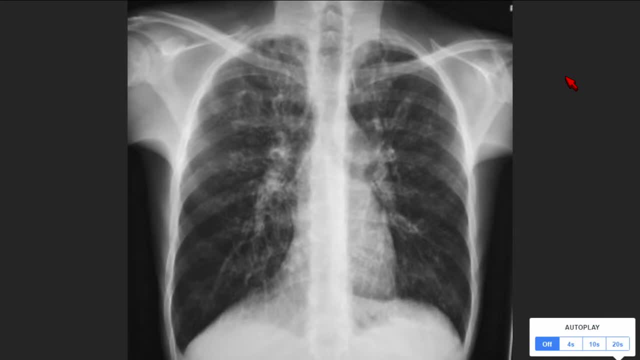 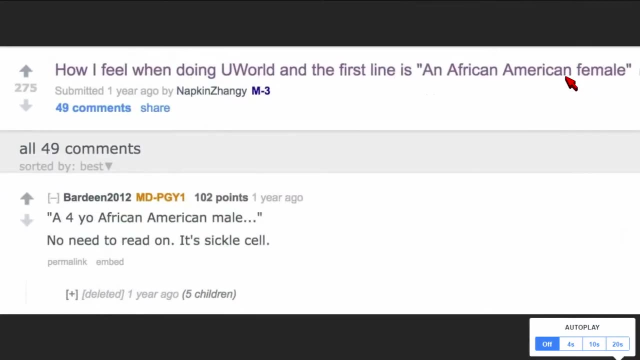 years of earlier intervention. It wasn't until race was effectively erased through radiographic film that doctors could assess her clinical picture accurately. Here's a picture from Reddit How I feel when doing UWorld, and the first line is an African American female. Do you guys know the UWorld? 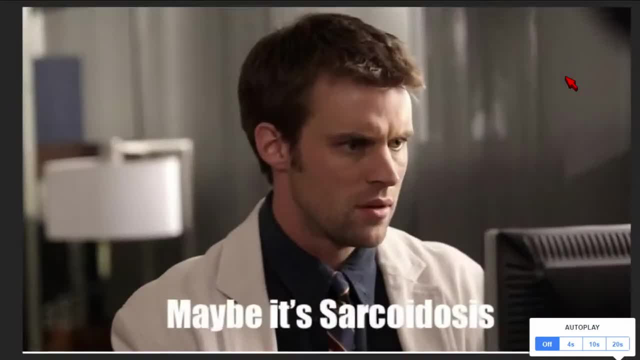 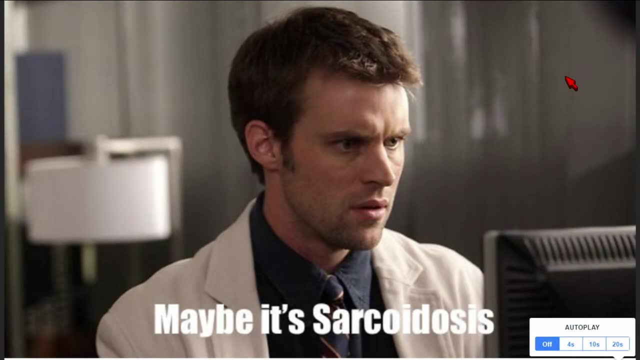 Do you have an idea what this might be? Sarcoidosis? Okay, so I think people had an idea of where it was going and it was literally from the words African American, female. No signs, no symptoms, there are no nodular whatever's. 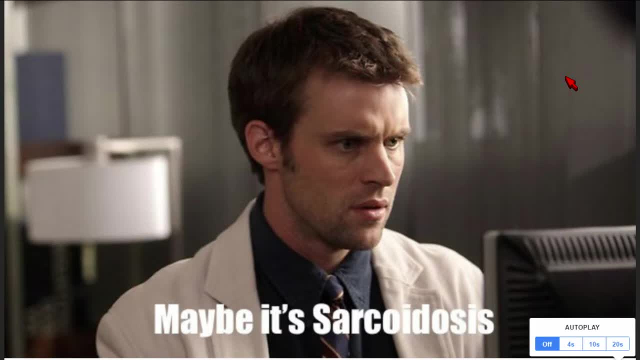 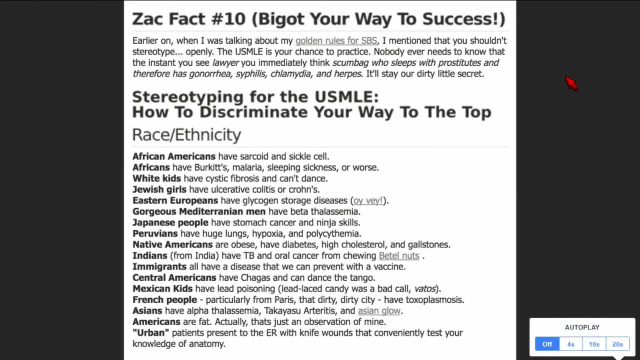 just literally from African American female. So this is a list to bigot your way to success. Here you're typing for the USMLE how to discriminate your way to the top Right. so I know these and it sounds like some of you know these. 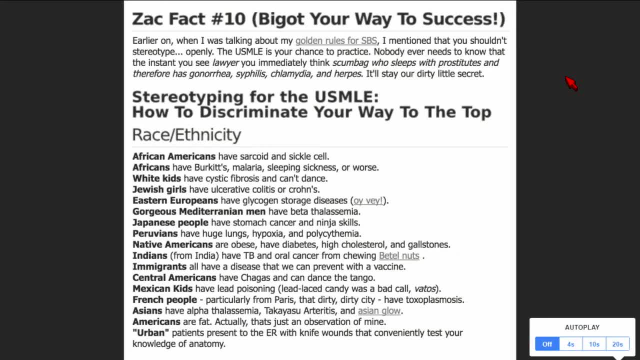 These are pretty slam dunk clues Right when you're studying for STEP. you will take anything you can get, So it really matters how students are taught. In 2013, a study by Phelan provided physicians with a clinical vignette that include either: 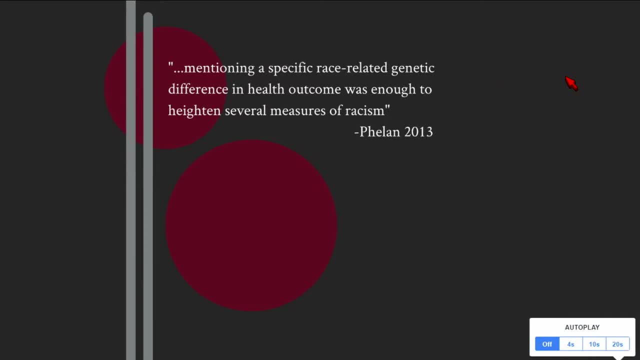 biologic or social race associations. It found that mentioning a specific race related genetic difference in health outcome was enough to heighten several measures of racism. Another researcher notes that persons who accept genetic explanations for racial differences tend to score relatively high on traditional measures of prejudice. 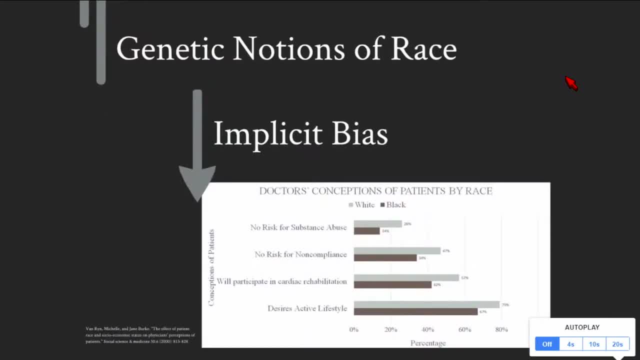 So thinking of race as biologic contributes directly to implicit bias in physicians. This has shown to manifest in differential expectations of adherence, non-compliance and risk for substance abuse. In a short story I was reading last year, I came across this line. 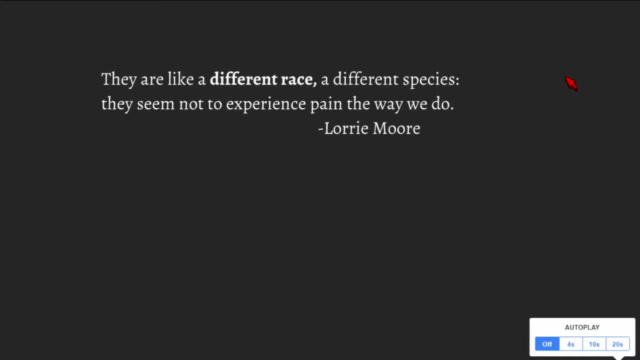 They are like a different race, a different species. They seem not to experience pain the way that we do. There is something within the public imagination that accepts fundamental biologic difference, And this trickles into clinical practice. I'm sure many of you have come across this data. 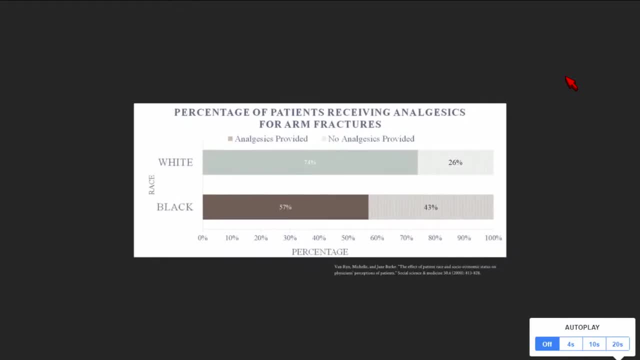 but black patients are almost half as likely to receive analgesics in the emergency department for long bone fractures. So this is: they've already been diagnosed with a humeral or femur fracture. Those are kind of painful, right Like we want to give. 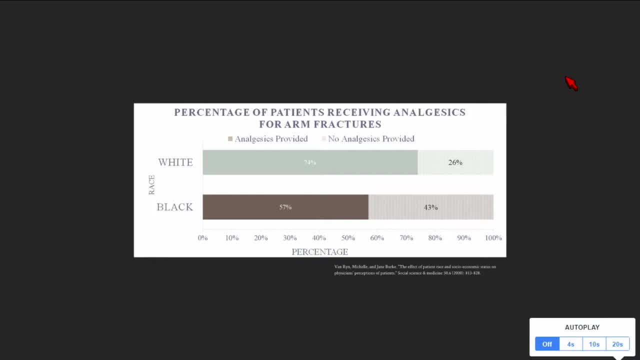 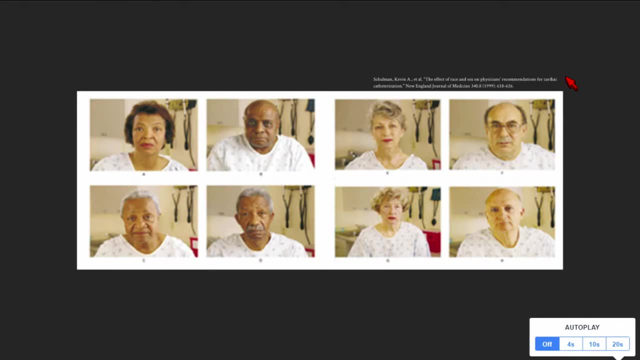 opioids to people who broke their leg bones. This picture comes from research that recorded physicians evaluating standardized patients who presented with a predetermined script describing cardiovascular symptoms. It concluded that our findings suggest that the race and sex of a patient independently influence how physicians manage chest pain. This supports other 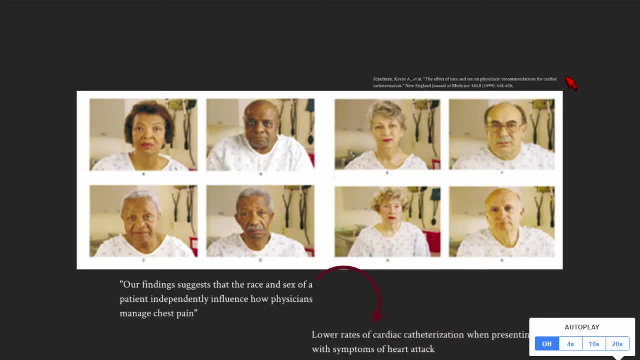 research that found that black patients had decreased rates of cardiac catheterization when they presented to the ED with symptoms of heart attack. Black patients have lower rates of every single type of organ transplant possible And, in fact, the only major surgical procedure that is more abundant in. 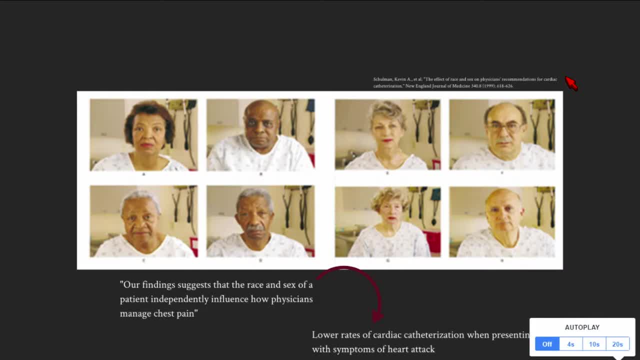 patients of color is limb amputation. If we are teaching race in a way that conjures, perpetuates and increases bias, this is a very serious thing to consider. And now, between delayed and unequal care, implicit bias and even beyond, regarding the larger picture of racialized inequality, 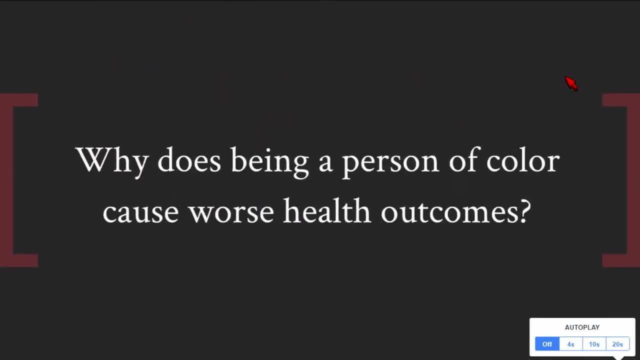 we're starting to see a bigger answer to this question. Why does being a person of color cause worse health outcomes? Again, what matters is how you ask about race, what you are trying to ask when you include race as a variable To make matters more complicated. 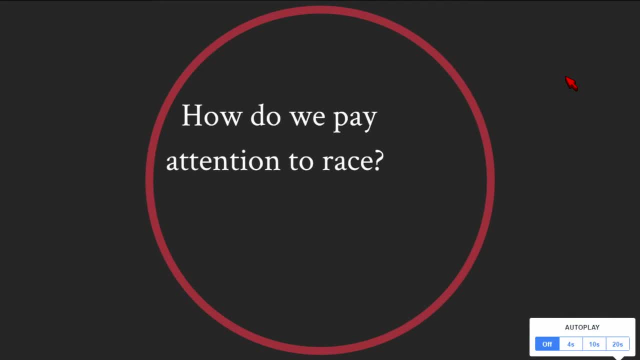 sorry. I feel like every time I transition, Abby was like: oh my god, you're using Prezi, don't make me dizzy, And I feel like I did it too much, so I'm sorry. I'm sorry, Abby, To make measures a little bit more complicated. 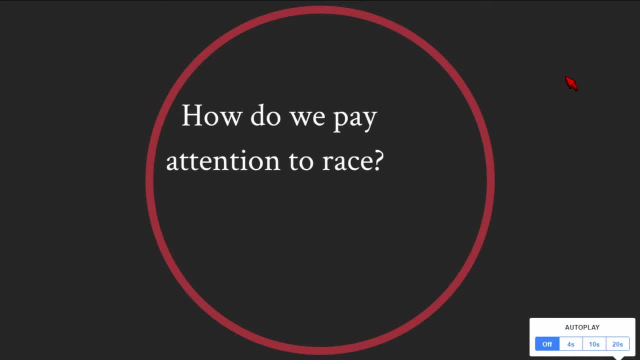 it's important to mention that mandating these racial categories in that 1993 Revitalization Act was seen as a progressive achievement. At the same time, as we noted before, emphasizing difference, especially biologic difference, implicates the idea that people of color are. 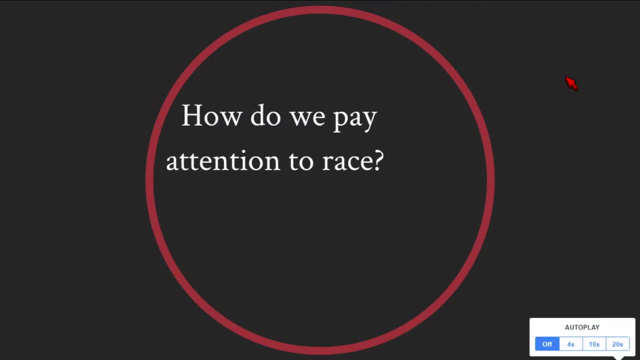 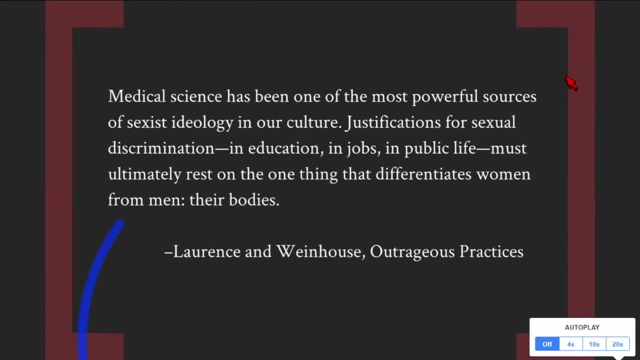 being dissimilar, So we need to pay attention to race, but carefully. This double-edged sword can also be seen in feminist movements. Women fought for inclusion in research studies in order to push for answers about differential presentation, reproductive health and drug efficacies in pregnancy. 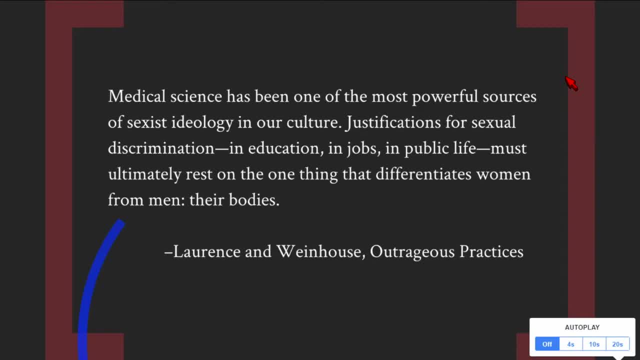 But at the same time, these efforts bolstered age-old notions that women are fundamentally, biologically different. So, at a time when you're fighting for justice by saying, look, equality is not the same as justice. we are not the same, we have specific needs. 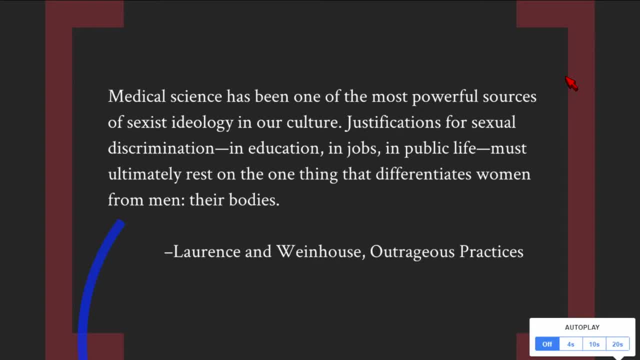 you're also kicking the can down the road and providing evidence that can be manipulated by people who say: look, this is proof that men and women are naturally distinct, naturally dissimilar, and therefore inequality can be realized as natural. And this validity of normalized 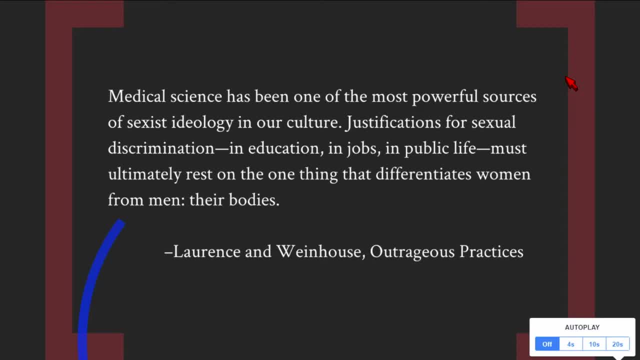 biologic differences between men and women or black and white people is not neutral. It's dangerous. It offers support when people like Larry Summers attribute low numbers of women in STEM fields to quote lack of intrinsic aptitude. It bolsters the idea. 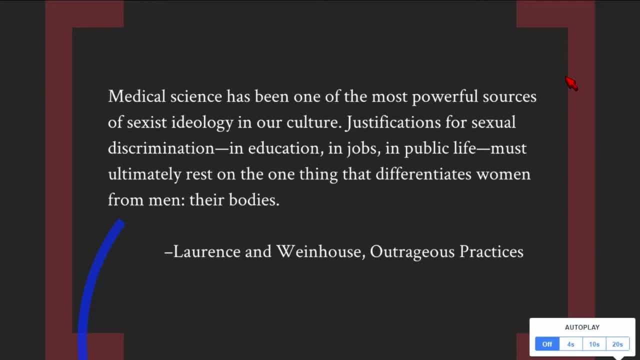 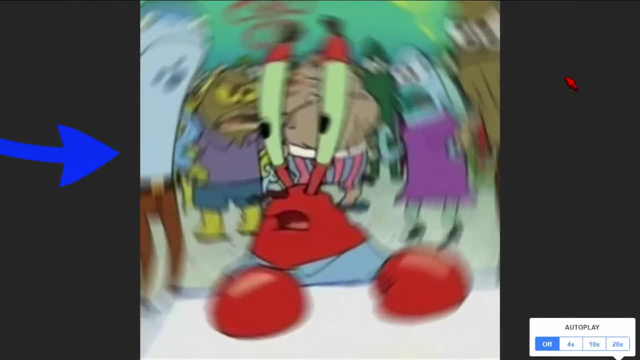 of genetic inferiority. It eclipses the weight of injustice At the end of the day. I know you want answers. There's a lot of mess when it comes to race in medicine, so what do I do? I'm sorry, I don't really know. 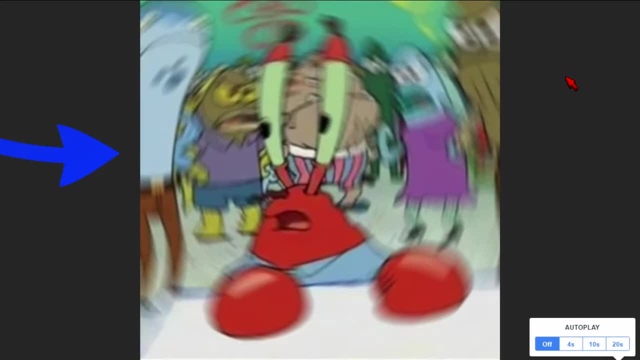 There's not a very clear answer, And I think it is really complicated, given that so much of our clinical knowledge and tools have already been built on racialized data. Add to that the fact that tackling race in the clinic is also very difficult, given how uncomfortable 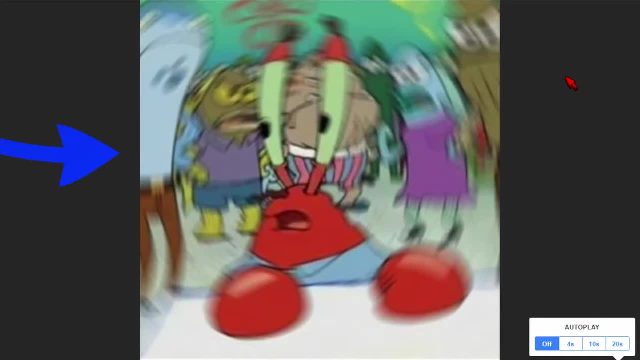 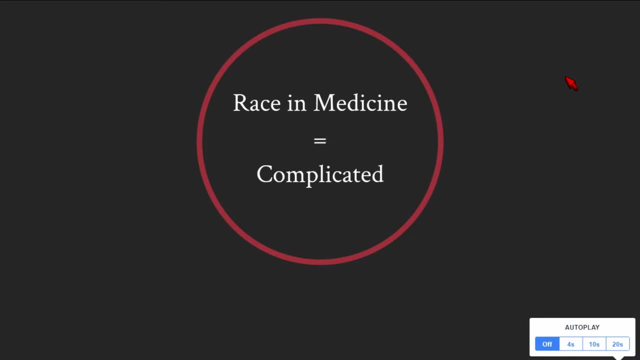 taxing and time-consuming it is to talk about. The only concrete thing that I do believe is certain that we cannot eliminate the discussion of race in medicine, no matter how fraught with discomfort it is. At the very least, we have to identify what the questions are. 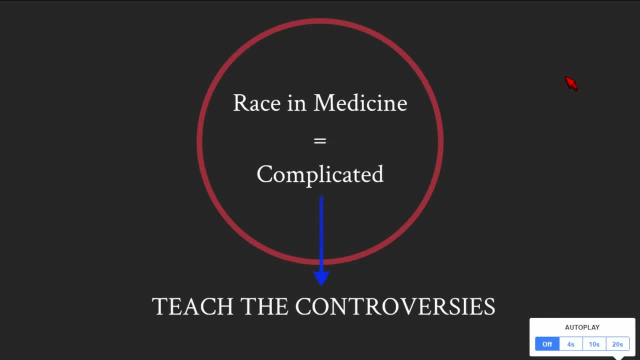 and we have to teach the controversies. So, even if we use race as a proxy in the clinic, we need to know how it is a proxy, its weaknesses and the risks that we run when we naturalize race-based medicine as a routine part of medical practice. 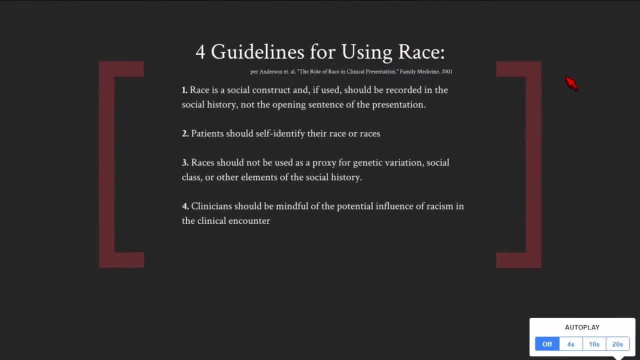 Because I do want to leave you with something concrete. Here are four recommendations for using race in the clinic, as suggested by Anderson et al in his paper The Role of Race in the Clinical Presentee. So one race is a social construct. 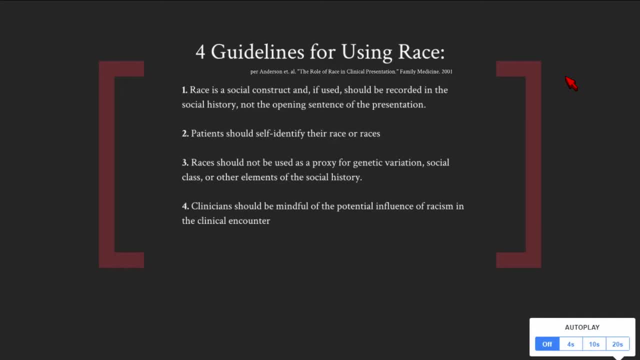 and, if used, should be recorded in the social history, not the opening sentence of a presentation. Two: patients should self-identify their race or races. Three races should not be used as a proxy for genetic variation, social class or other elements of the social history. 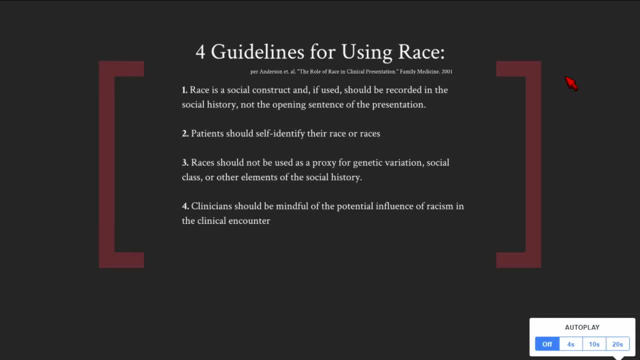 Four clinicians should be mindful of the potential influence of racism in the clinical encounter. Using race in clinical practice is really complicated, and what it comes down to is: as a clinician, what do you learn when you look at race? What does knowing race teach us? 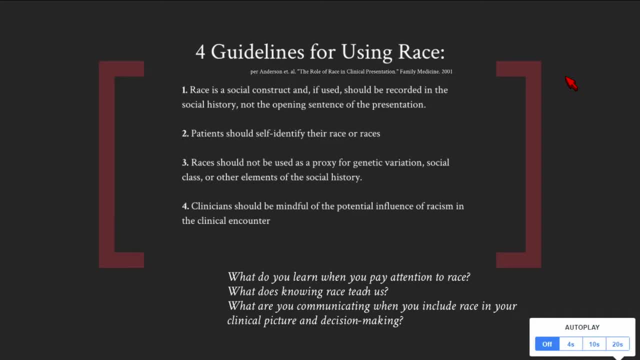 and what are you communicating when you include race as part of the clinical picture? A lot of what we say in the emergency department is unspoken. So if and when you include race in your note, in your oral presentation, pay attention to why you reached for it. 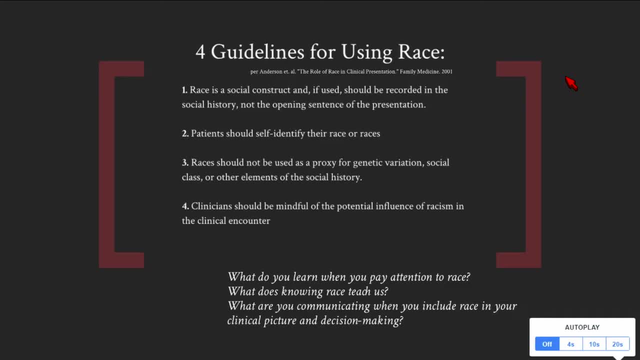 Are you using race as a proxy for cultural identity because you think diet matters? Do you actually know what the patient is eating? Are you using it as a substitution for social class to conjure a certain picture? Did you write it because you wanted to be aware? 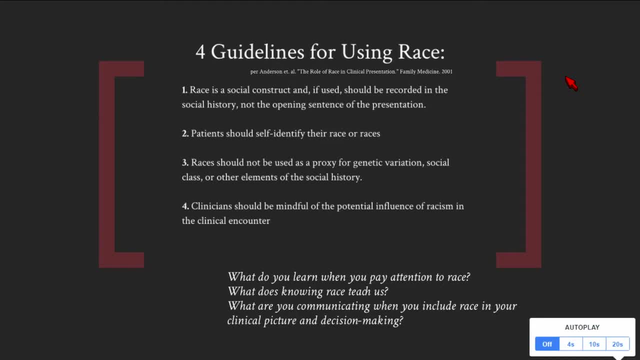 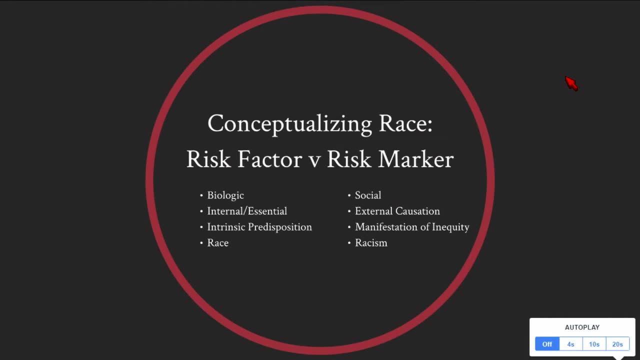 of iatrogenic harm during their hospital stay. I think a quick way of summarizing this is to explicitly recognize race not as a risk factor, which is often portrayed as an internal biologic variable that drives disease predisposition, but as a risk marker. 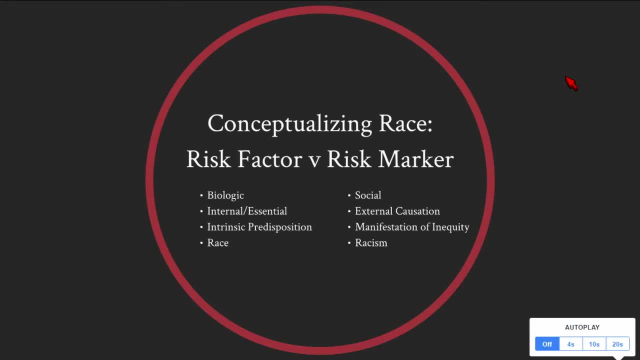 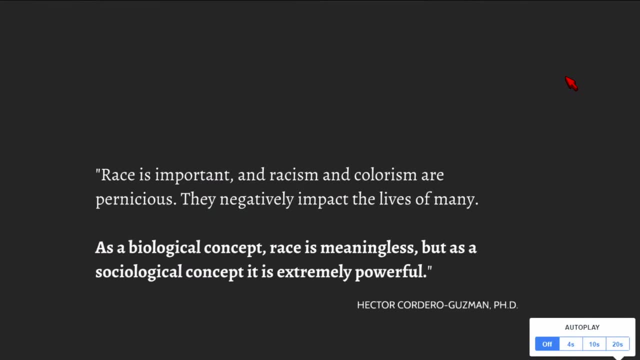 which invites harm as a consequence of racism. Before we end, there are two main takeaways that I want to repeat. So one: I think a lot of people get stuck on this idea of race being a social construct because they interpret it as implying that 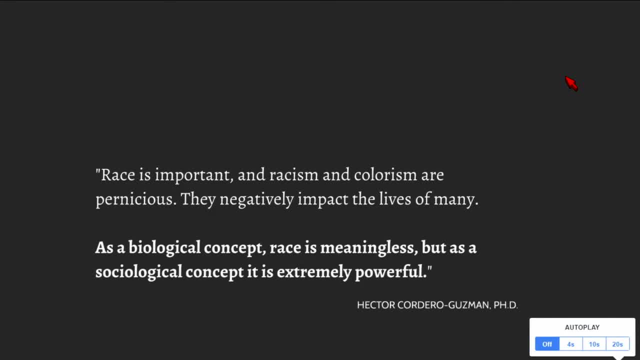 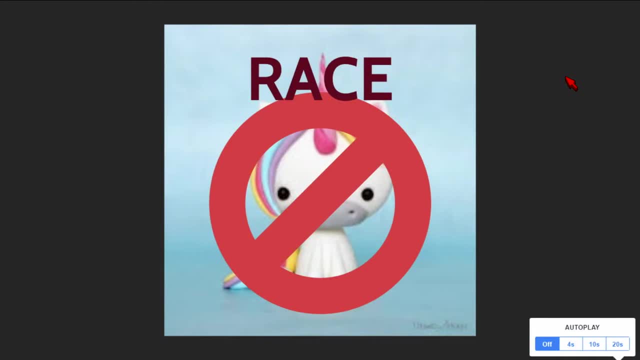 race is made up, so it doesn't matter, And I want to reiterate that race is not a unicorn, It is a social construct, but it doesn't mean that that's unimportant. It is indeed a category that is culturally engineered, but it is a category. 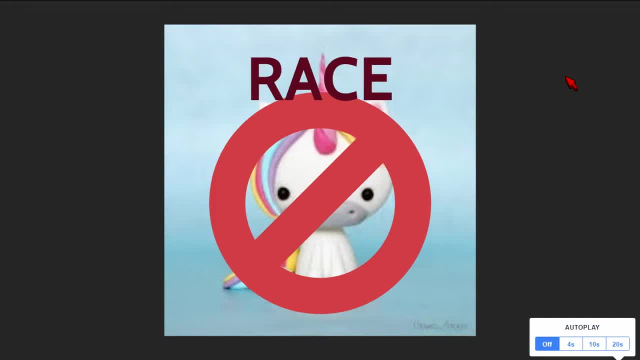 that is still meaningful, and abundantly so, given the data that we've seen on racial discrimination in multiple venues. Additionally, saying that race is a political category rather than a biologic category does not mean it doesn't have impacts on biology and health: Diabetes, hypertension. 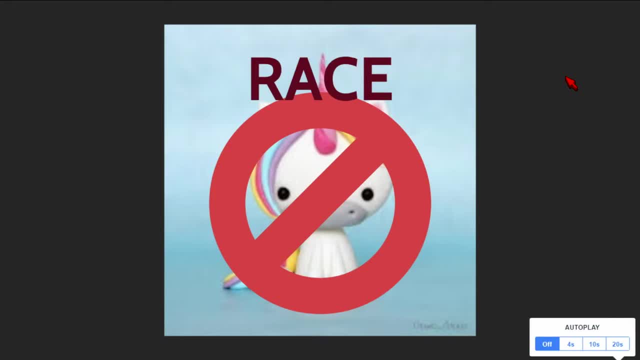 myocardial infarction. these are all pathologies caused by inequity. They are biological consequences to a social ill, even though race is a political idea. In medical school we had a lecture on sickle cell, where we learned about the extreme pain of sickle cell crises. 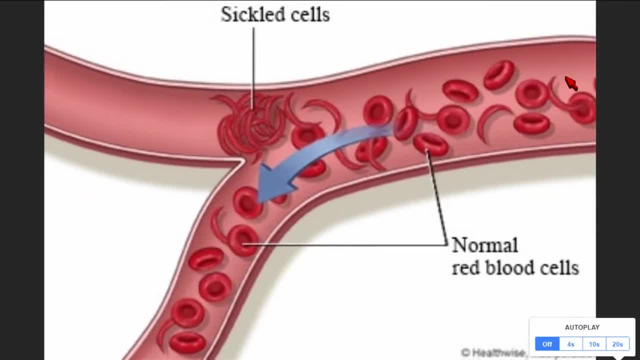 As you guys know, there are no lab results or tests that can readily demonstrate that a patient is experiencing a crisis, And at the end of class our lecture minimized her presentation and stepped out from behind the podium to give us one last sort of lesson, and I think 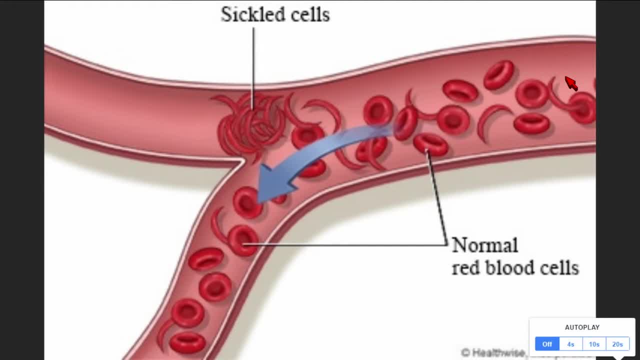 it was the most important lesson that she gave us. She told us that she explicitly instructs her black patients that, no matter what kind of excruciating pain that they are in, before they go to the emergency department they must do two things. 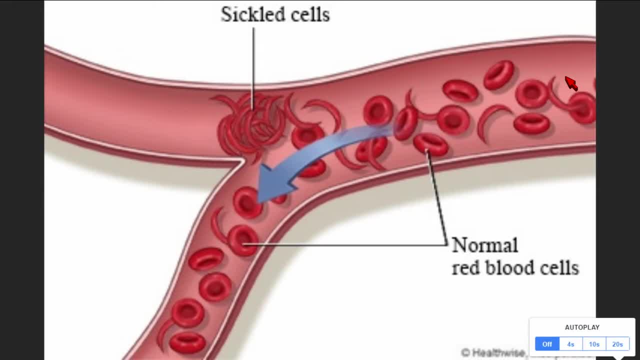 They must one shower and two dress in business casual clothing. In other words, they must act as if they are headed to a job interview. They must present themselves as trustworthy candidates. She knows that. otherwise their chance of receiving adequate pain management in the 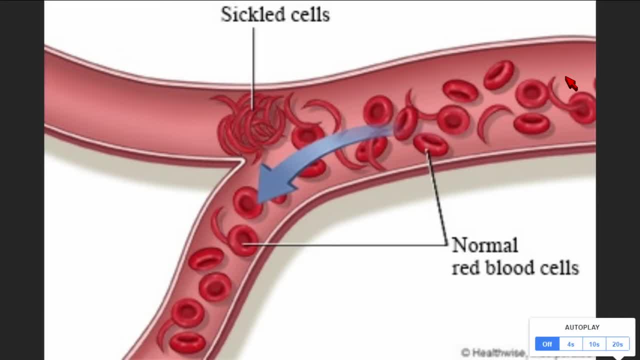 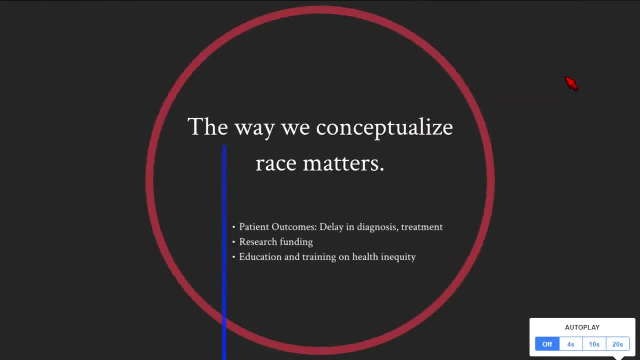 emergency department is significantly reduced. So race is made up, but it's not a unicorn. It has very significant repercussions. Second, I want to reiterate the way that the way we conceptualize race really does matter. It's not just about technical. 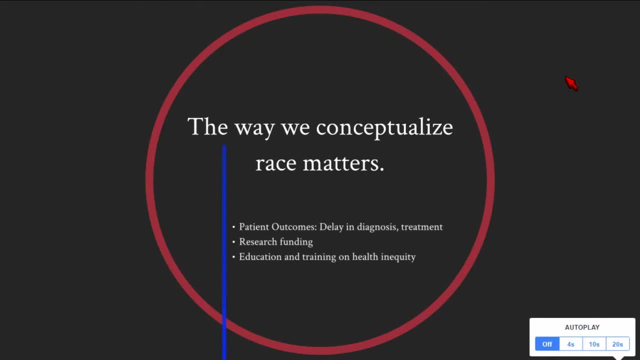 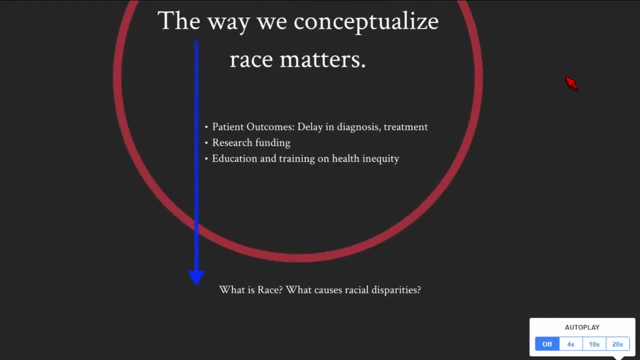 definitions or squabbling over semantics. Being accurate about our comprehension of race and health inequity can save lives. The stakes are very high. The first question of this presentation was: what is race? The question is important because the word race appears so often in front of the words disparity. 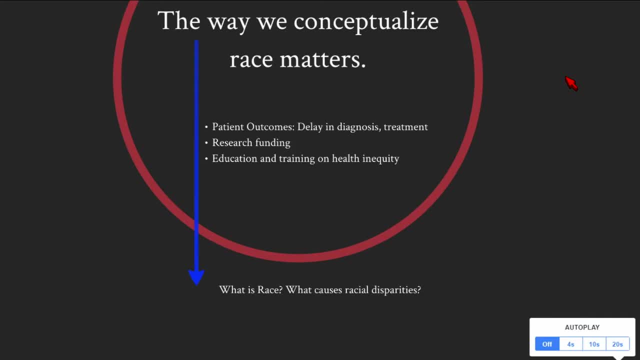 inequity and inequality. The way we answer shapes our entire theories about the causes, sources as well as solutions for sickness. in our country, All throughout medical education and training, we are told implicitly and explicitly that race is genetic, innate, essential and 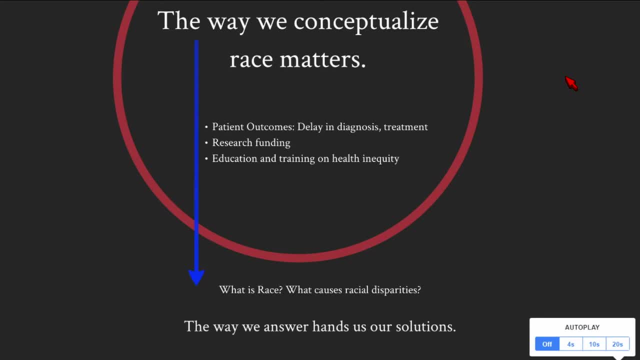 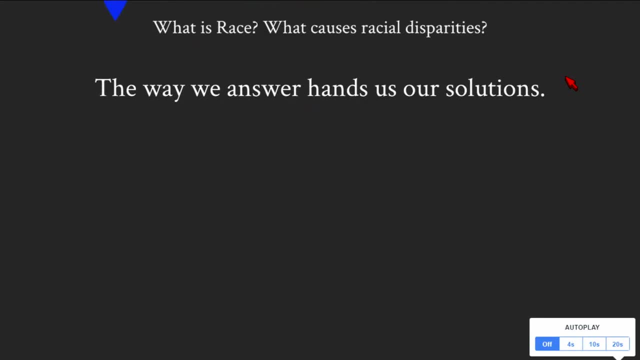 physiologic. This belief is rampant in our house. But consider alternatives. As Chris Chen notes in his essay, The Limit Point of Capitalist Equality, on the one hand, race is a form of culturalized stigmatization and misrepresentation requiring personal 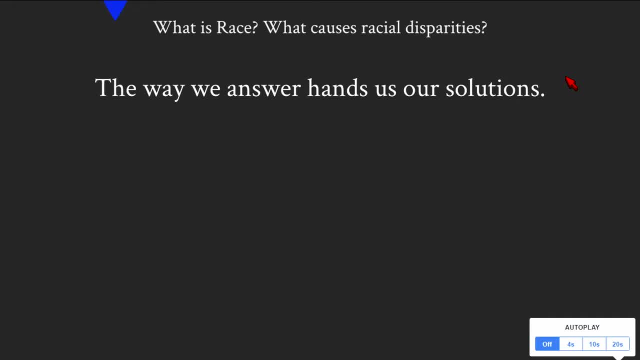 institutional and or state recognition On the other. race is a system of wage differentials, wealth stratification and occupational and spatial segregation. If racial health disparities can be reduced to physiologic and genetic phenomena, the answer to our ill health is relegated. 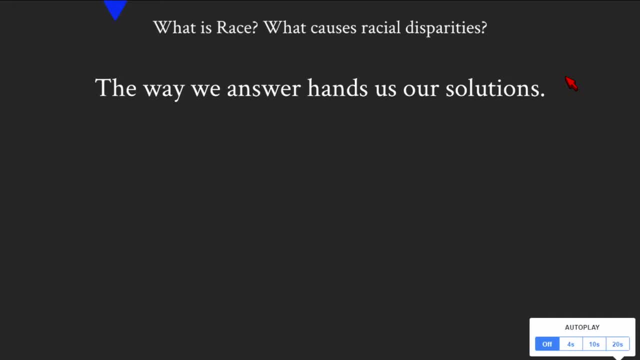 to technological advancements and biologic interventions. We don't need the March on Washington or fair housing or the vote. We need pills, genetic therapies, maybe some diversity training. We don't need community activism, We can simply buy the products and the services. 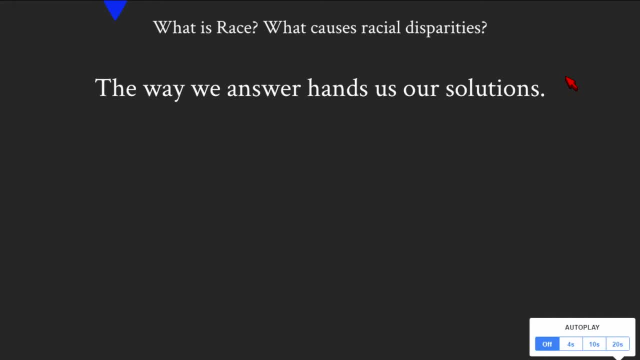 that we derive from our biomedical research. The way we answer these questions also tells us about culpability. So when you look at racial inequity, where do you see the flaw? When you look at these health disparities, when you see this 100,000 person gap, 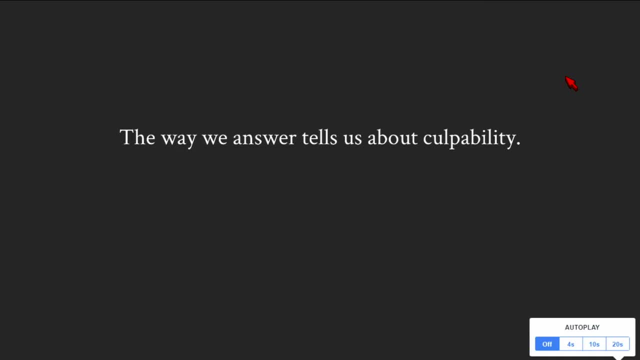 in survival between black and white citizens in this country. do you really and truly believe it is because of innate black failure? Recognizing racism as the linchpin of health inequity changes the conversation. The culprit is not difference, not genes. 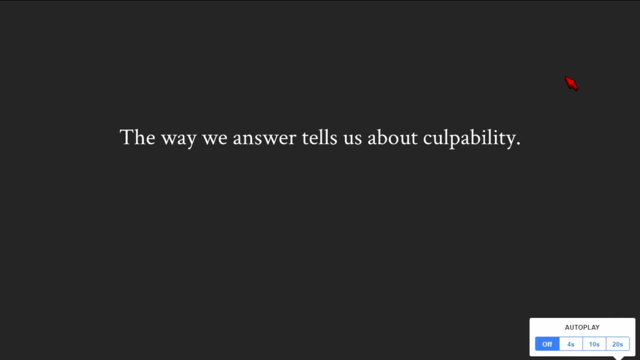 but supremacy. There is a tremendous opportunity in medical training and practice to rectify problematic thinking about race, biology and difference. A really compelling way to think about it comes from an article by one of my heroes, Nancy Krieger. She's an epidemiologist at 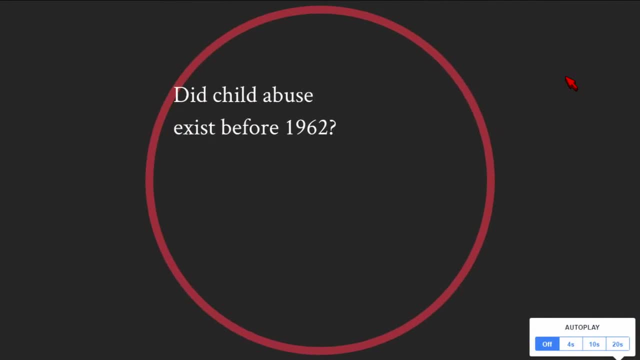 Harvard School of Public Health. So Krieger asks: did child abuse exist before 1962, when C Henry Kemp and co-authors published the now classic article The Battered Child Syndrome? Certainly, she says, Did child abuse harm health before 1962?? 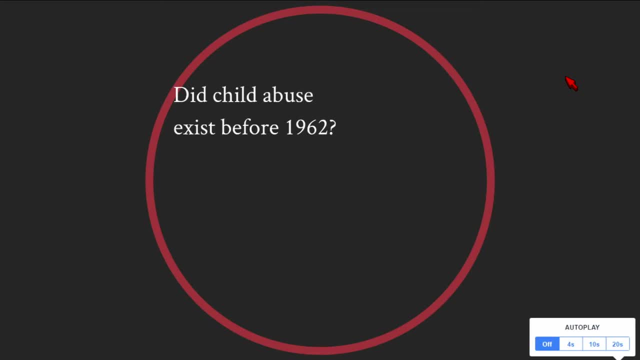 Of course, But before Kemp's article gave it a clinically recognized and medically legitimate name. child abuse was not a part of American medical or public health agendas. This name Battered Child Syndrome offered a volatile societal problem validity as a serious health issue. 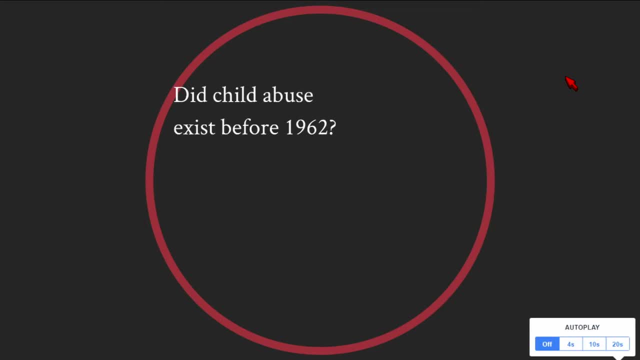 It was no longer a hushed secret or unspeakable shadow, a nebulous shame with no edges for purchase. Child abuse was concretized as a threat to health that could be rigorously scientifically and institutionally documented and monitored. Doctors were taught to screen identify. 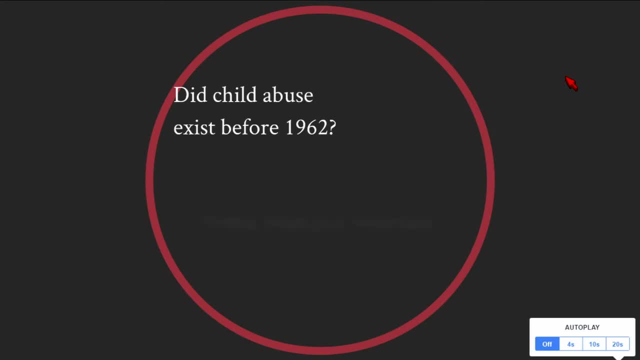 treat and care for its victims. Similarly, naming racism gives us purchase The ability to recognize it, offers a path for explicit investigation, and the identification of racism as an enemy of public health signals its deservedness as a recipient for major attention as well as major resources. 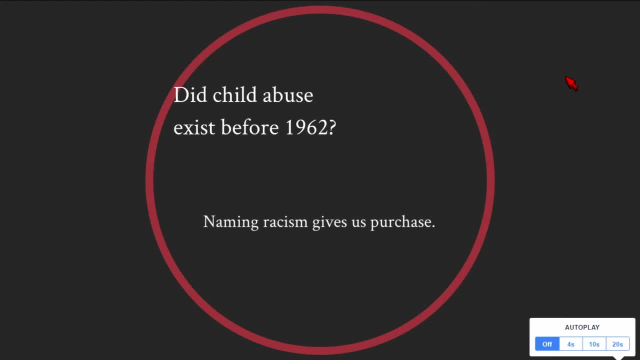 When we encode work, education and research as anti-racist, we conjure in our collective imaginations a way to render the violence obsolete, Like child abuse. naming racism now does not mean it did not exist before. It is not, as Krieger says. 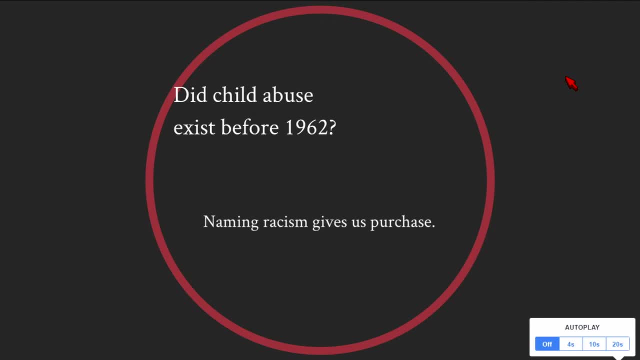 novel to suggest that health is harmed by heinous crimes against humanity, such as slavery, lynching, genocide, and also by the grinding economic and social realities of everyday racism, Though the problem has existed for centuries. she says the serious scientific study of racism. 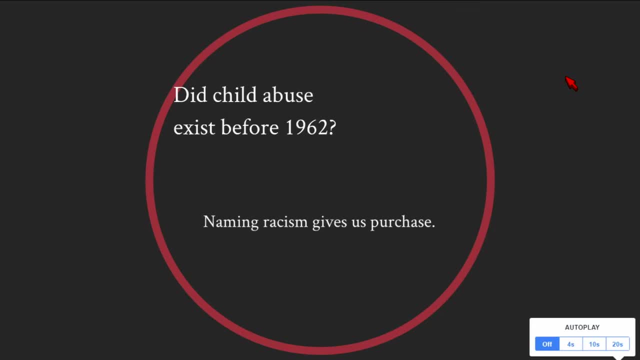 as a determinant of population health remains in its infancy. We in academic medicine have the opportunity to change that. At the beginning of this presentation, I offered a quote from Adichie's Americana. What's the deal, doctors in the house? Is race an invention or not? 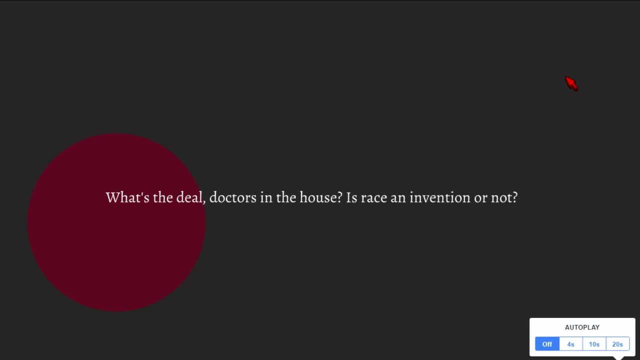 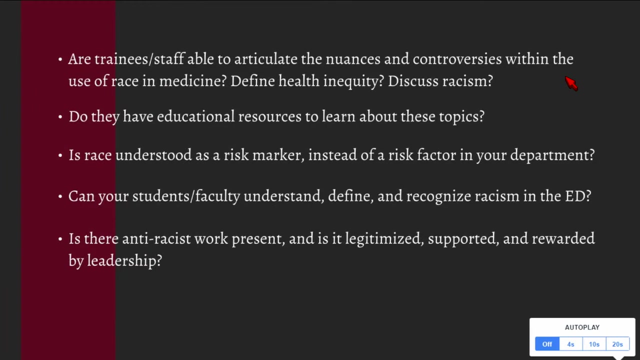 She asks this and directs the question because we are expected to know. I think a lot of this again comes back to education. So, when it comes to thinking through your training program or accreditation, are trainees or your staff able to articulate the controversies within the use of? 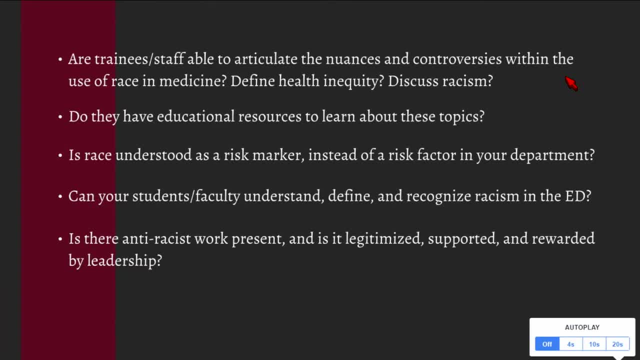 race in medicine? Do they have educational resources to discuss and learn about them? How is race understood as a risk marker and can your faculty understand, define and recognize racism in its own house? Is there anti-racist work present and is it recognized, supported? 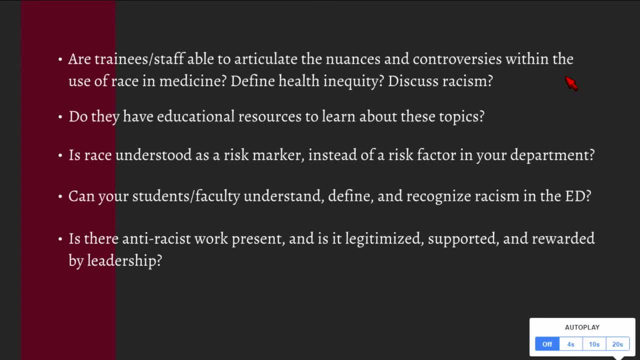 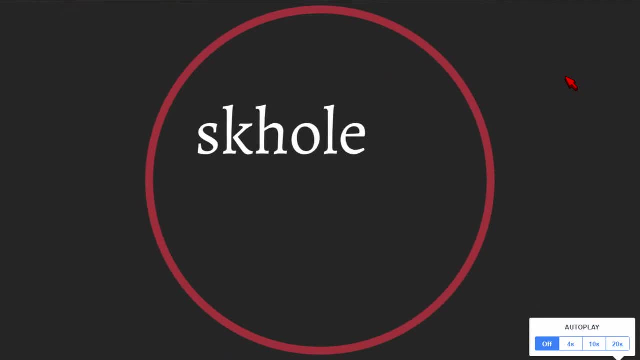 and in fact rewarded by your leadership. But it also can't be just about ACGME compliance. Benjamin Honeycutt, a historian at the University of Iowa, makes the point that the word school comes from the Greek word for leisure. He says. 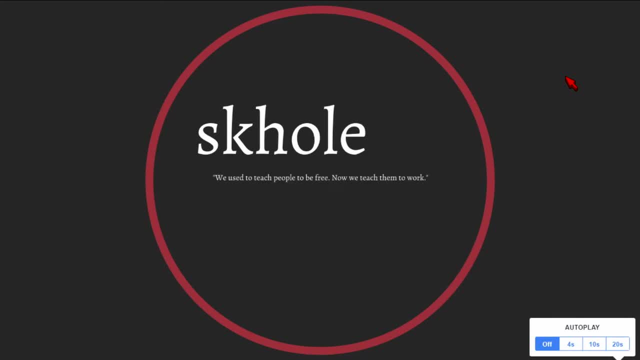 we used to teach people to be free. Now we teach them to work. We've all witnessed and experienced moments when the work of medicine keeps ourselves and our patients from being free. Hospitals and healthcare systems, like any and every institution, are vulnerable to the same powers. 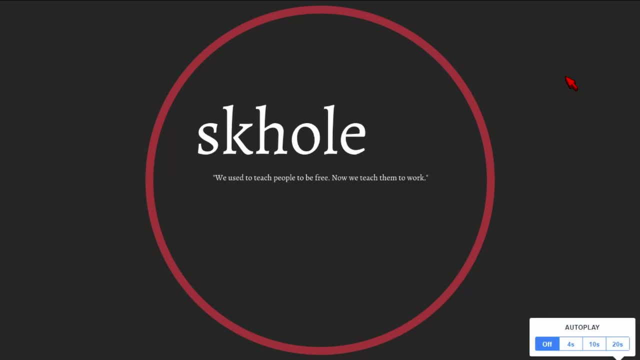 that create inequity. Supremacy is easy to cloak in words such as efficiency and professionalism. I am passionate about the subject of race in medicine and I am passionate about education because I truly believe it matters. I believe it sets the stage for our understanding. 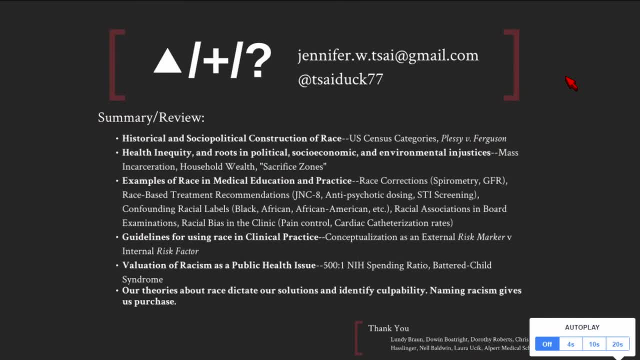 of the world. Thank you. I don't know how much time we have for questions, maybe we don't, But also that's my contact information. Please feel free to send questions or feedback. I am always interested in improving this presentation and this conversation. 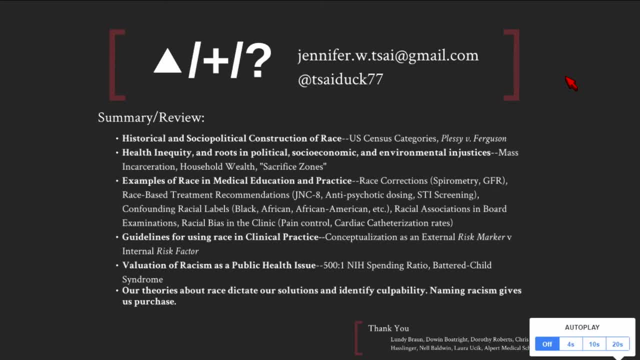 So your input is really appreciated. Another question: What do you think about the biological explanation for hypertension being more common in African-Americans where, because of like slave ships and water retention and things like that, there's a biological explanation for hypertension being more common in African-Americans? 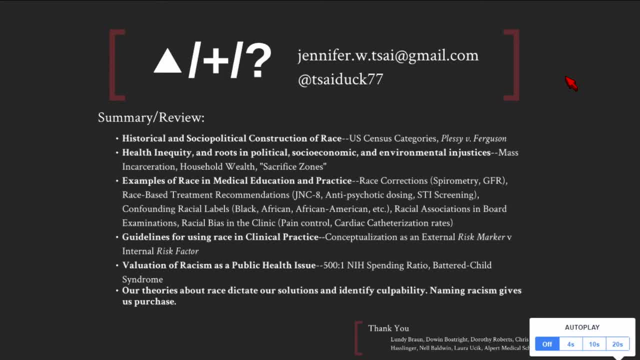 where, because of like slave ships and water retention and things like that, there's a biological explanation for hypertension being more common in African-Americans. where, because of like slave ships and water retention and things like that, there's a biological explanation for hypertension being more common in African-Americans.